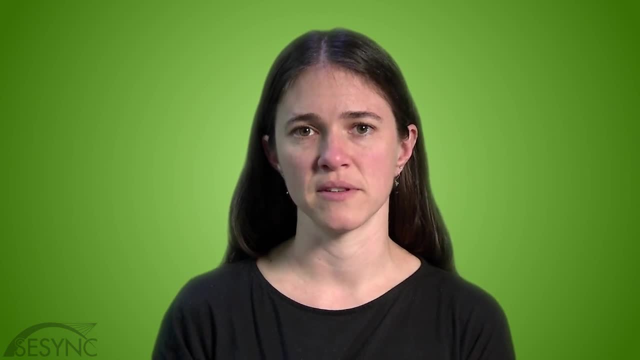 He notes that population dynamics can be characterized by the null hypothesis of exponential population growth and that any other dynamics can be explained by factors including cooperation, competition, interspecies, interactions and resource limitations. He highlights the concepts used to measure these factors, including discrete time models. the Allee effect. 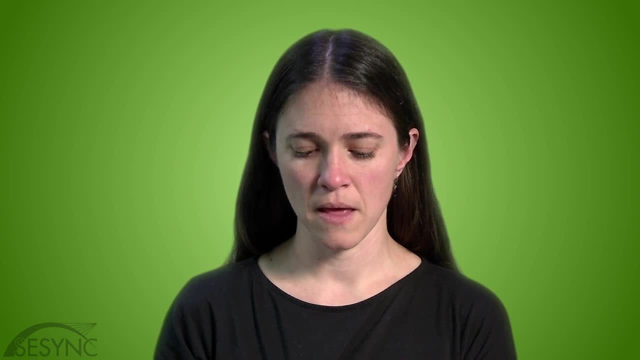 positive and negative density dependence and carrying capacity. He concludes by noting the data challenges associated with modeling density dependence in a population and also notes that population dynamics and factors that influence those dynamics will change over space and time for a given population. The first part: 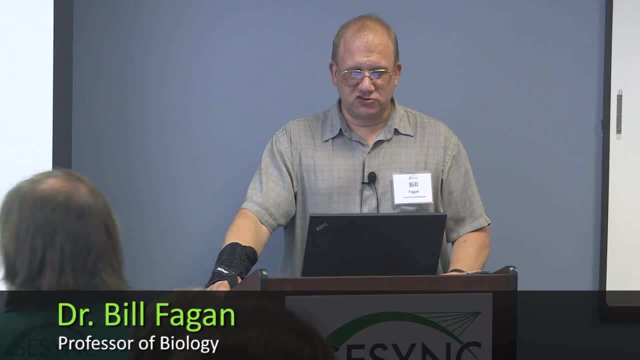 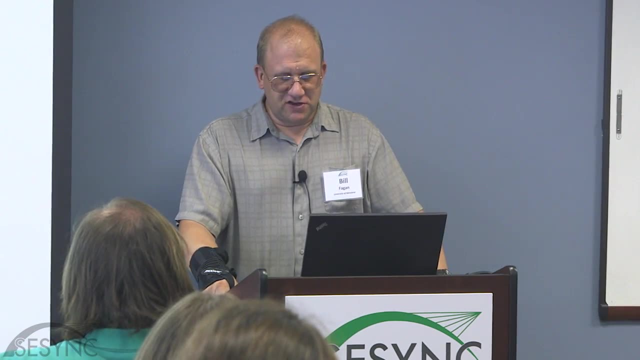 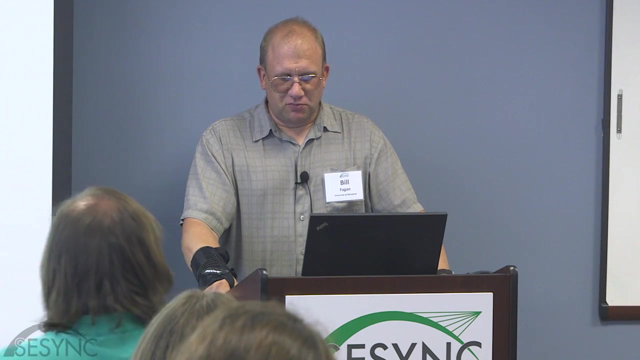 of the talk will be on core principles of population growth, just to try to introduce to folks who are not coming from a strong background in ecology some of the key issues that are of interest to ecologists interested in population dynamics. Then I'm going to move on to spatial problems and methods for modeling those spatial problems in ecology. 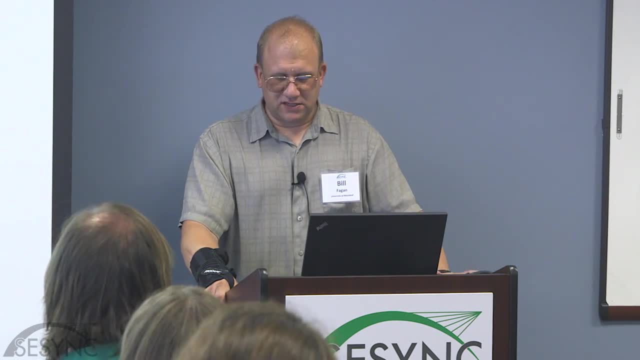 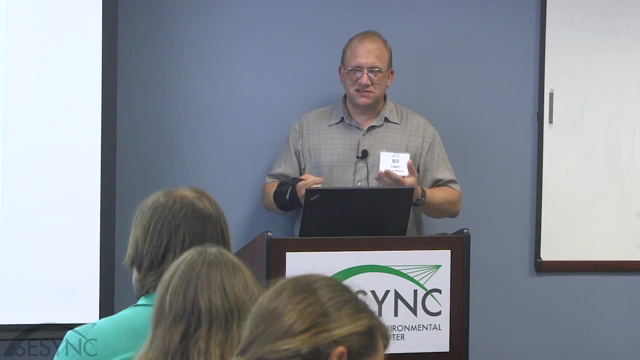 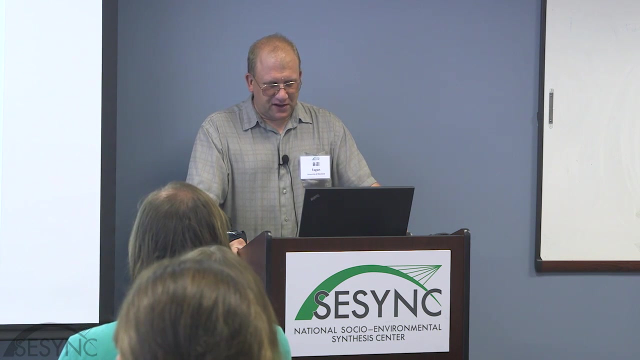 and try to show a little bit of the diversity of the toolboxes that are out there available for tackling spatial problems. And so what socio-environmental issues does any of this connect with? Well, actually a lot, And so these are some of the topics that I thought of that connect quite tightly to this interface between population and spatial ecology. 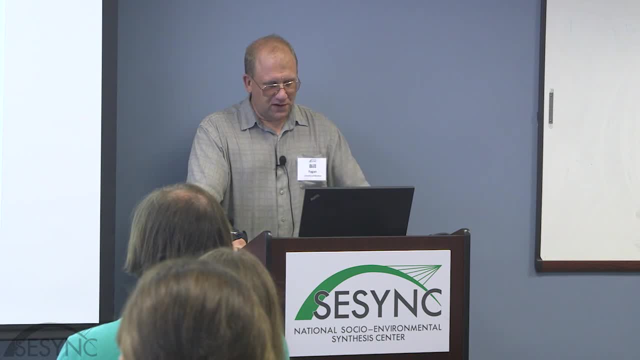 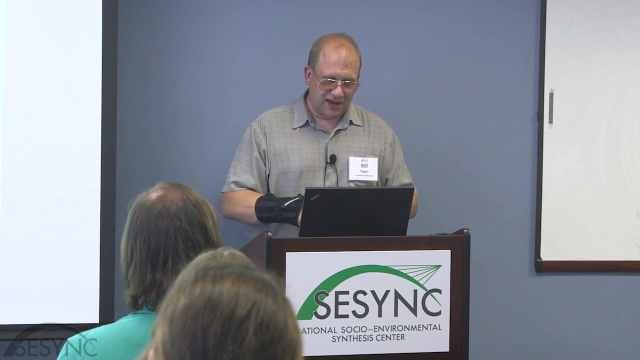 Fisheries, invasive species, which we'll hear more about tomorrow from Dan Simberloff- biological control- I'll talk a little bit about that today- questions of ecological footprints and also conservation and reserve design. All of these things Hinge upon key issues of population dynamics and how they play out in space. 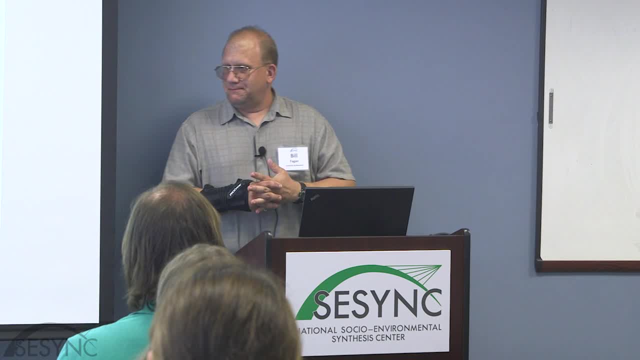 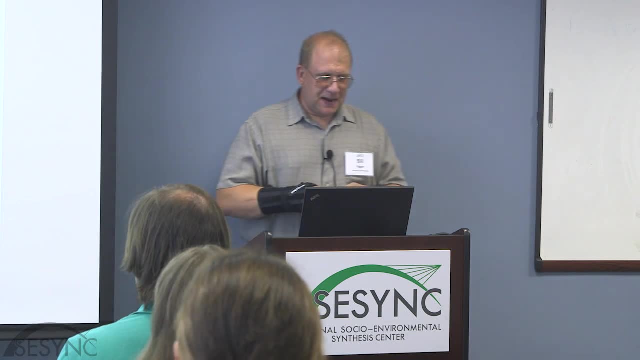 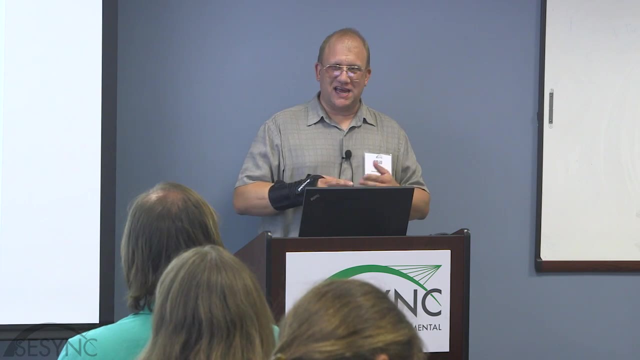 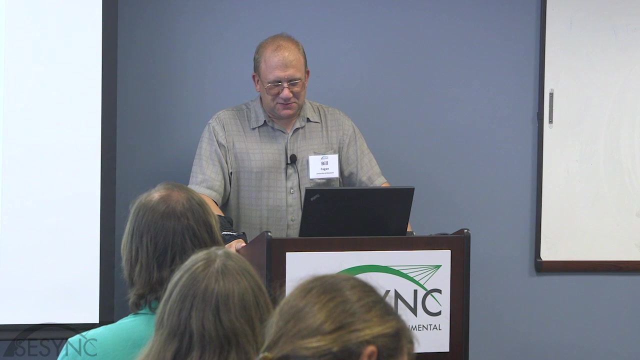 So one of the readings that was assigned as a sort of a succinct foundational document is this paper by Berryman, where there was something of a lament that ecology needs to have general rules and principles, like in physics for example, And this paper identified a series of five such basic principles. 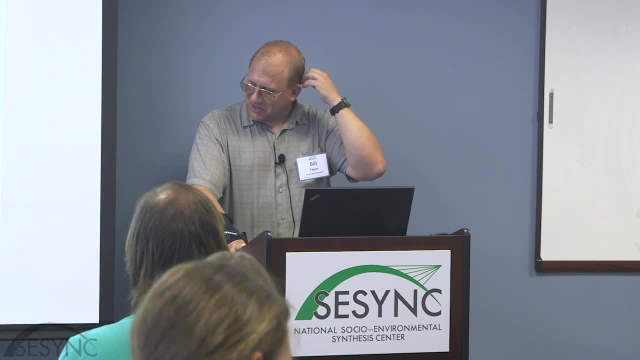 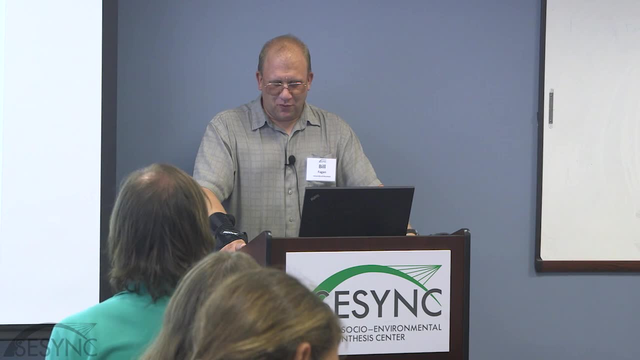 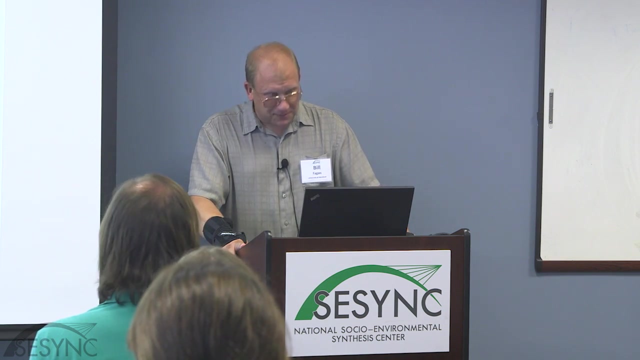 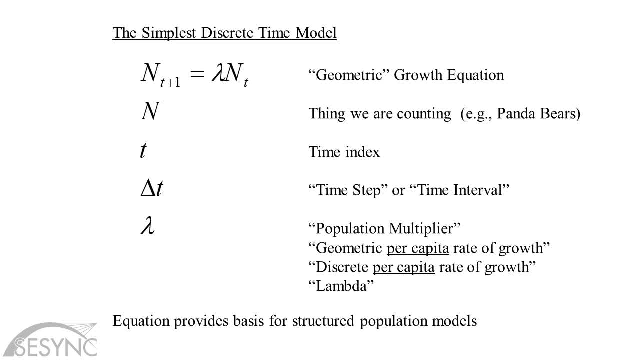 And the question becomes: if you don't have exponential population growth, what causes the deviation from that null baseline? And these are the different definitions of the elements in the model. And these are the different definitions of the elements in the model. This thing here, the time step or the time interval, is implicit in the way this is written. 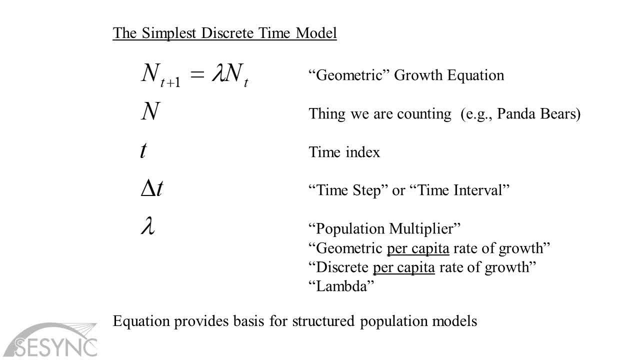 This thing here, the time step or the time interval, is implicit in the way this is written, And the key piece here is our parameter—the population multiplier, sometimes called the geometric per capita rate of growth or the discreet per capita rate of growth or some. 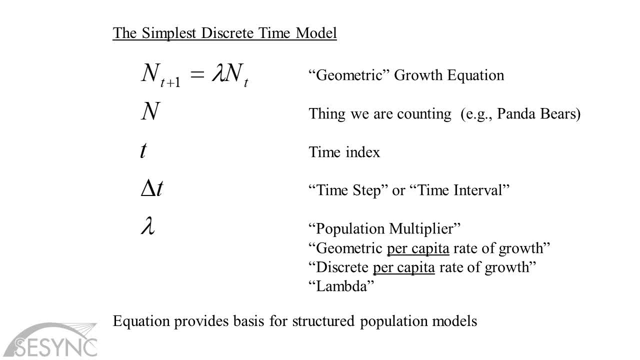 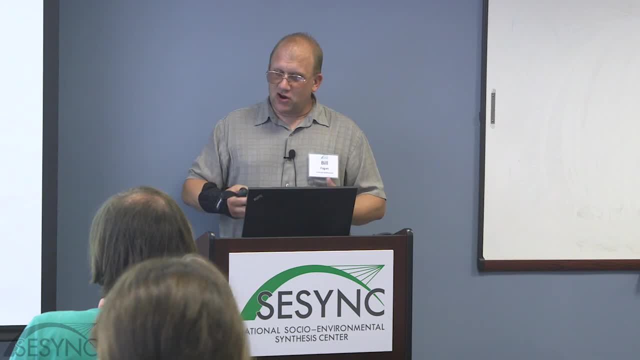 people just call it Lambda, and it's kind of universally known what this refers to, and this kind of a set up provides the foundation for much more complicated models that have other kinds of biologically specific optimizations and animals that do very butterfly-like facts. 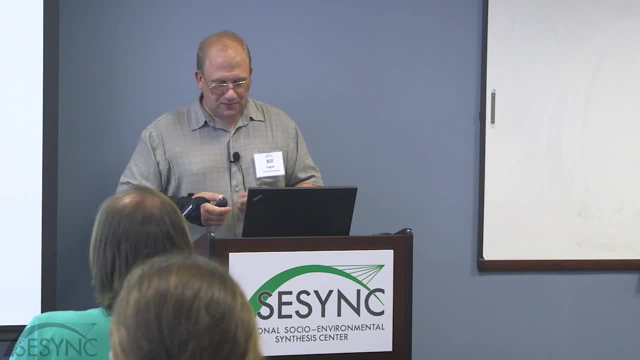 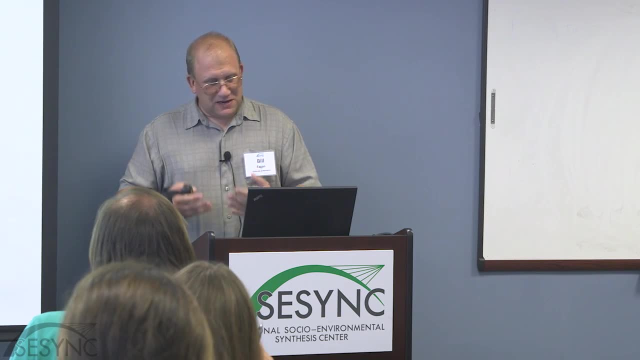 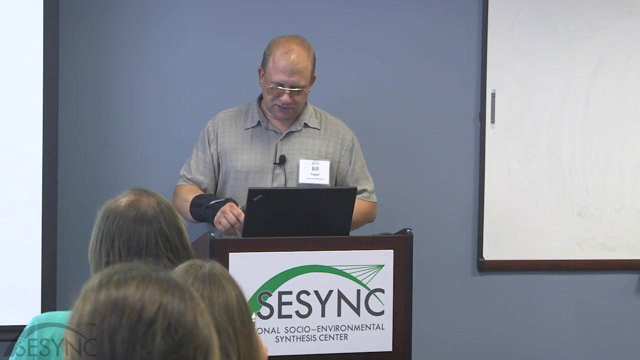 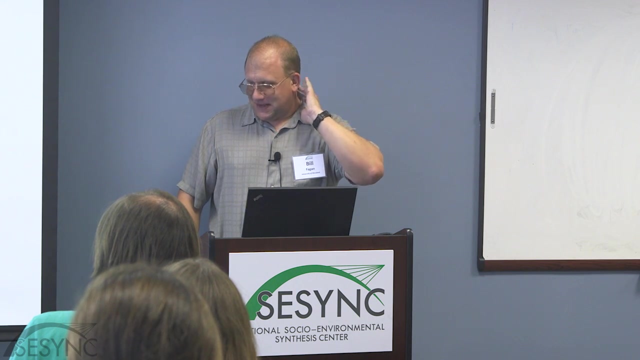 details captured in them, such as structured population models that demographers or people that are familiar with sort of epidemiology or human demography kind of questions would recognize quite nicely as bridging from social systems to human systems, to ecological systems. So if we're thinking about the connection to the kind of box setup that Wendy had talked, 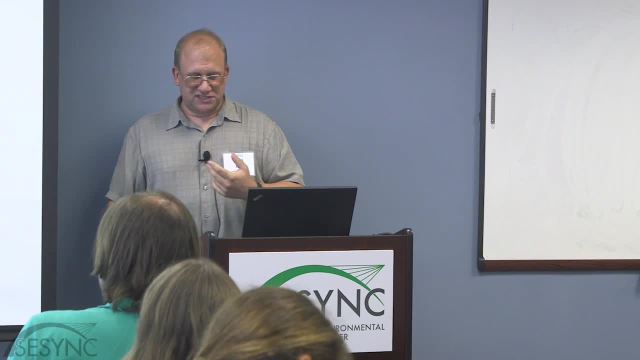 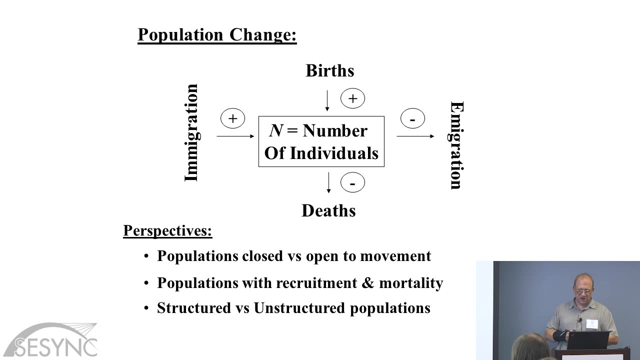 about earlier. we can think about population change in the same way. We can define what our box is, the census pool, the number of individuals that live in there. that's our population, And we can think about changes that are happening to that population. 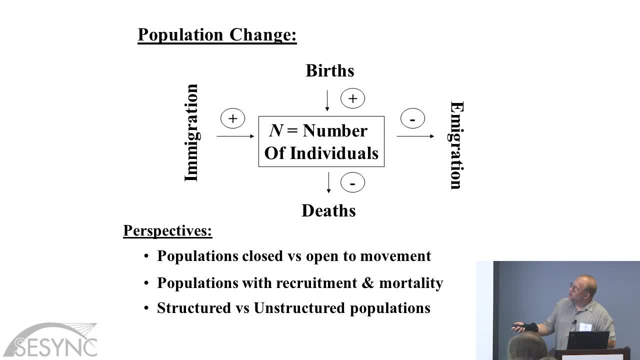 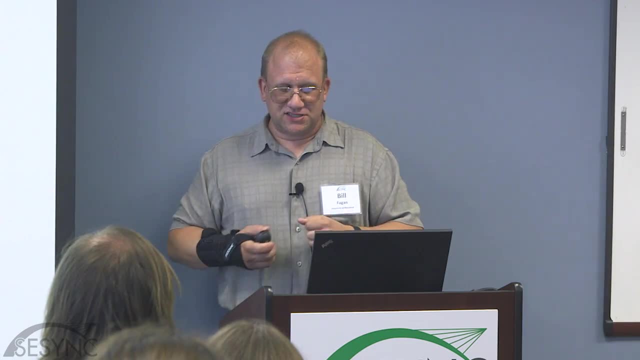 We can have individuals that are being born and added to it, or individuals that are immigrating into that population, also adding to that local population, And we can have losses through emigration Or through death. And so this kind of a setup, this boxiness, allows us to think of a sort of a starting. 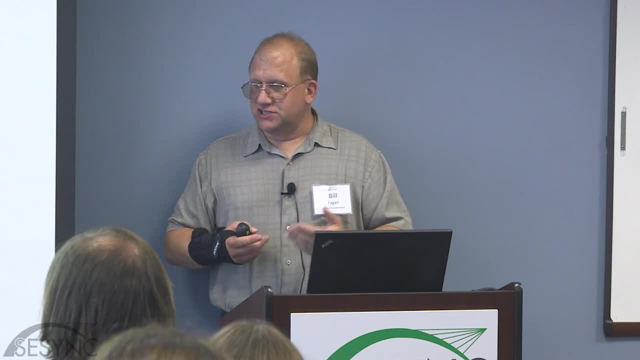 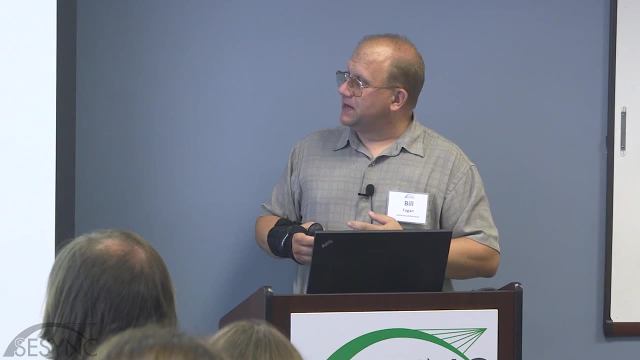 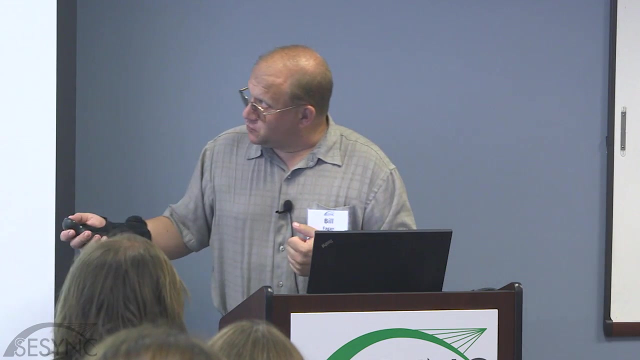 point for adding additional complexities. We can have populations that are open or closed to movement, such as the things I'll talk about later when I start talking about spatial models. We can have populations that have recruitment and mortality taking place, which would be situations where we're focusing mainly on this vertical axis. 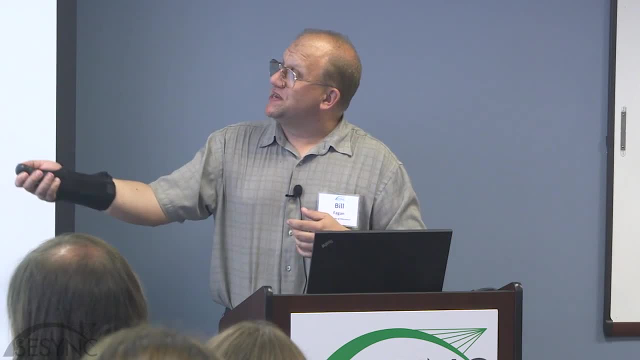 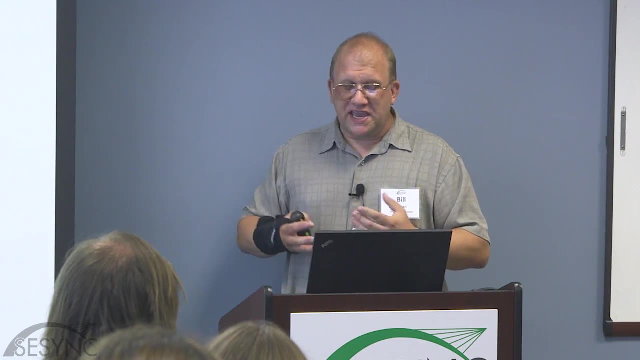 Or we can have structured versus unstructured populations, which is when we take our box and we start subdividing it in different ways. So these are kind of different tweakings that we can do to this starting platform to think about changes in population size. 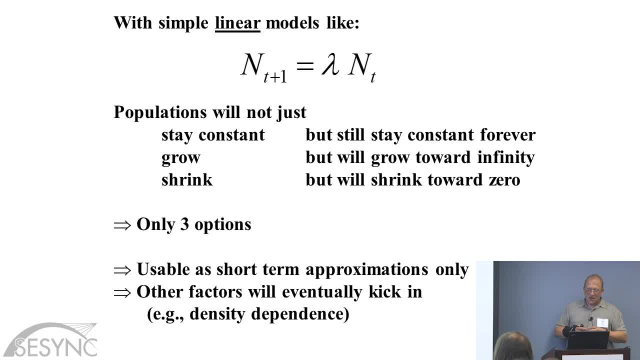 Now, if we have a simple linear model like this, we'll only have three options for what that model might do. The population will not just stay constant, but if it has a lambda of one, it will stay constant. It's going to stay constant forever. 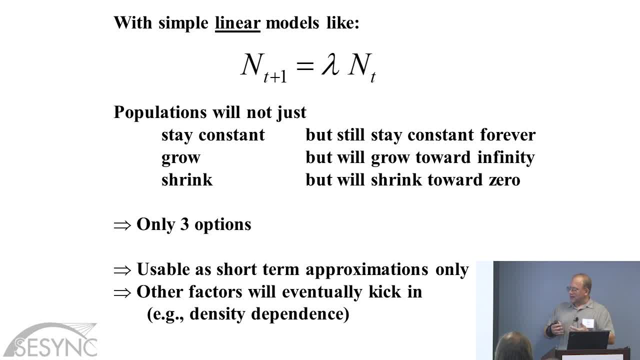 If lambda is bigger than one, the population will grow, And not just grow, but grow toward infinity, forever. And likewise, if the population has a lambda less than one, it will shrink towards zero. There's only three options with this simple kind of model. 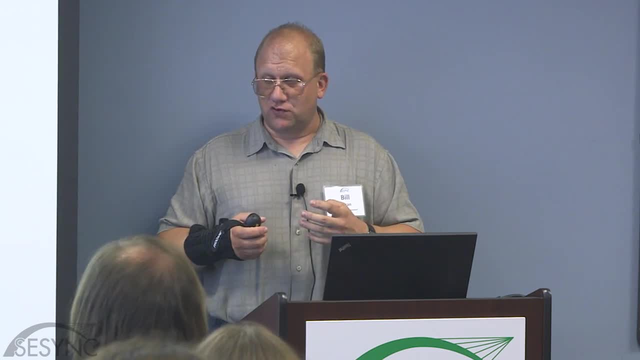 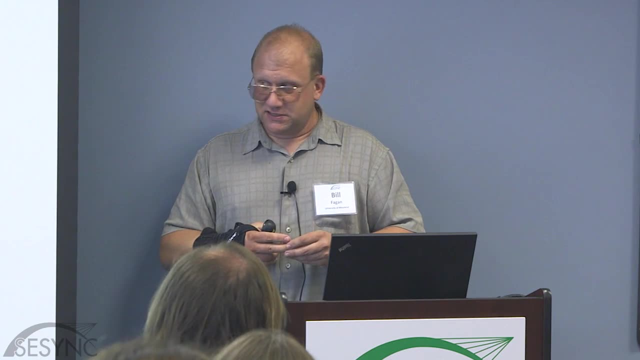 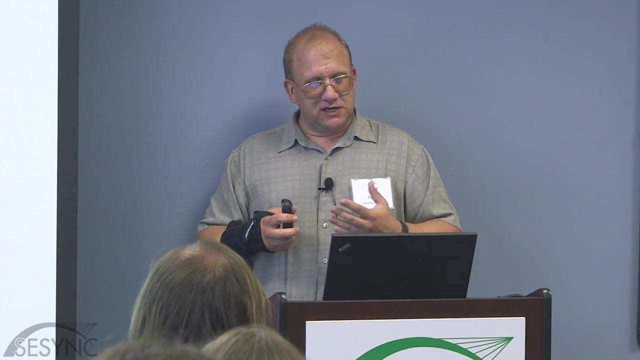 And so, therefore, this kind of simple model is only useful as a short-term approximation, Because other kinds of factors are eventually going to kick in, one of which is density dependence, Like Brian mentioned. So this is the first principle, that exponential population growth provides a null baseline. 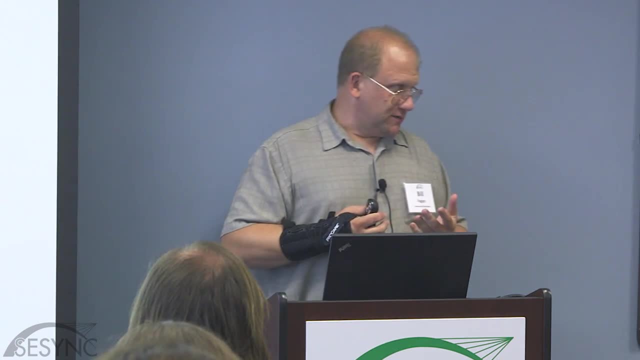 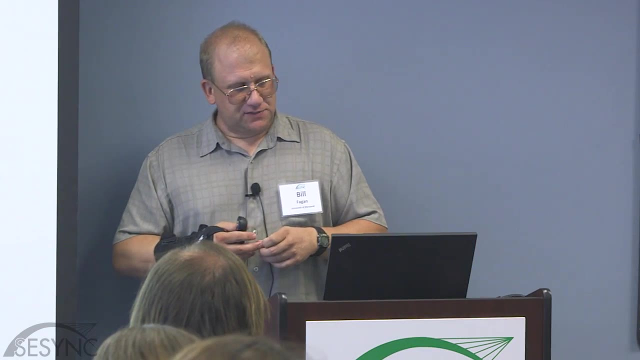 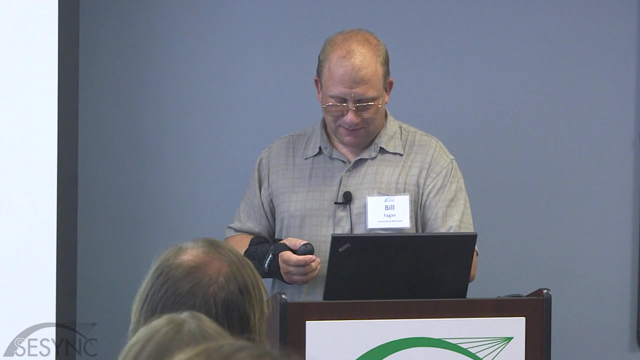 A second one is the idea that there can be cooperation among individuals. This is one deviation, one way in which real populations might deviate from this notion of exponential population growth, And this brings up what's called the Alley Effect and is an example of a threshold response in a population. 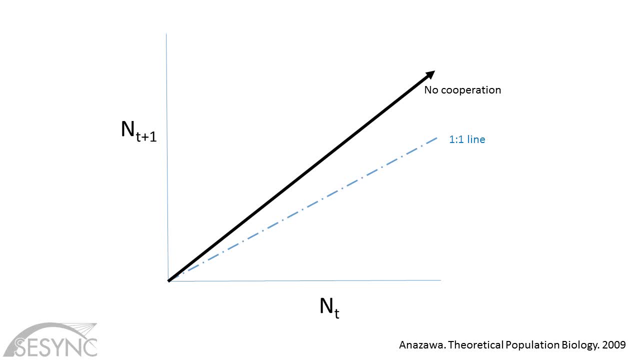 So if we have a population and we want to graph out what's happening, I'm going to borrow heavily from this paper by Anazawa here, because it has really nice graphics for trying to convey this kind of idea. So here's our population in year t. 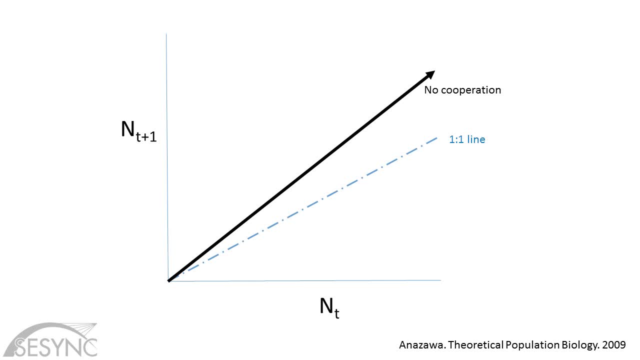 And on this axis is the population in year t plus one, And the blue dotted line gives us a one-to-one relationship. That simple linear model that I talked about is the line in black, That's the no cooperation model, And the slope of that line, how high it is, how far it deviates away from that one-to-one. 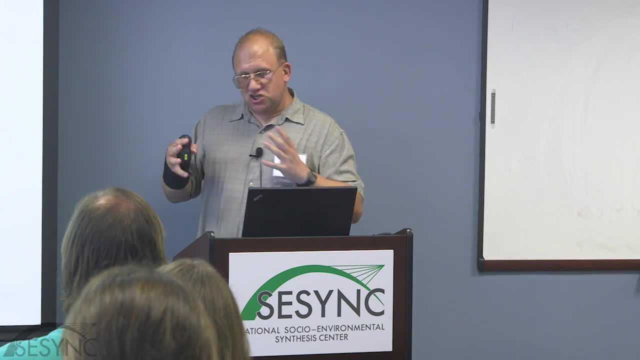 is our measure of lambda. okay, So this is where there's no interaction among the individuals. Everything just multiplies from one year to the next And there's no effect of density in any way. But if we go on, we can have different kinds of cooperation showing up. 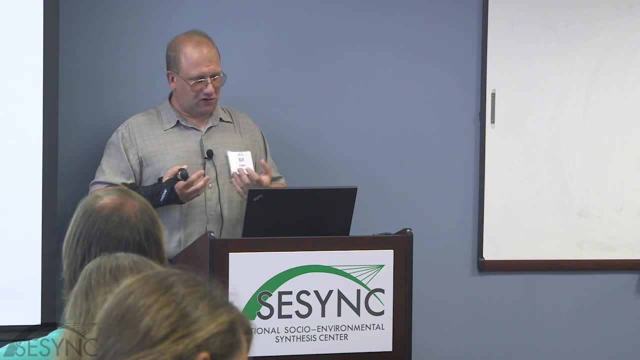 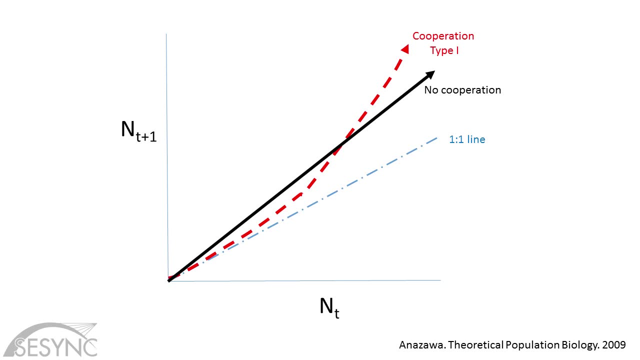 that represent some details about how individuals interact with one another. Here's one example of this. This is one kind of cooperation And you can see here it starts to deviate immediately from the from a linear relationship, And that you get an increase, that the magnitude of the deviation increases. 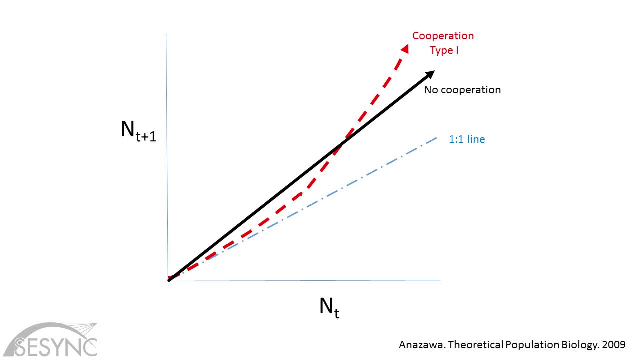 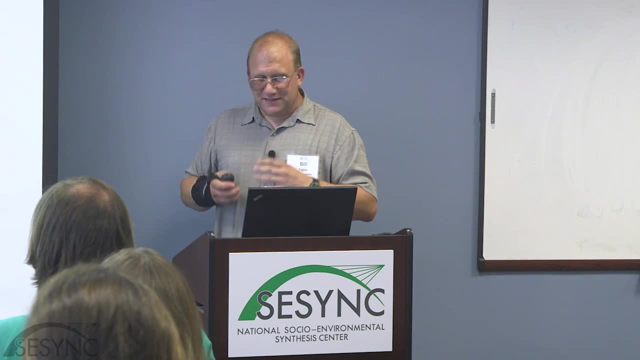 as the population size gets bigger and bigger, The deviation away from that one-to-one line gets larger and larger. The same kind of thing can happen under a different model of cooperation, But there's this difference that's quite subtle in some cases but quite important from the perspective of dynamics. 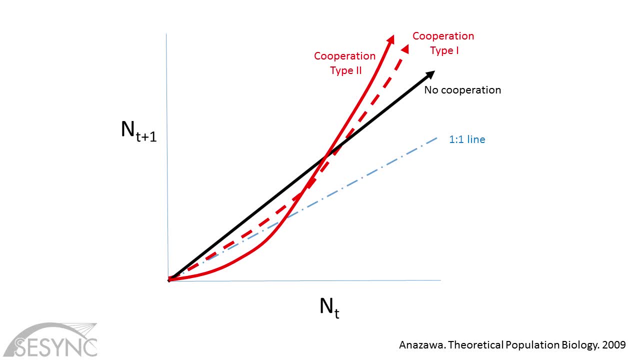 So you still have this idea. You still have this idea of a curved shape that is hinging on the notion of individuals cooperating with one another in some way, But there's something different about it. It's here where I've highlighted with this circle: 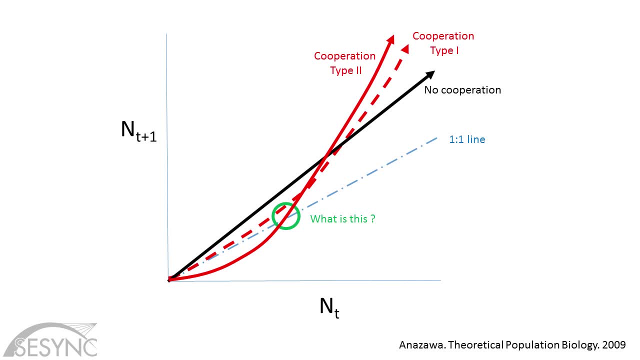 What's going on where I've put this circle, where the red curve is crossing the one-to-one line. What does this mean graphically? How do we intuit that? What's going on? There's some kind of critical threshold in population size which, if not attained, 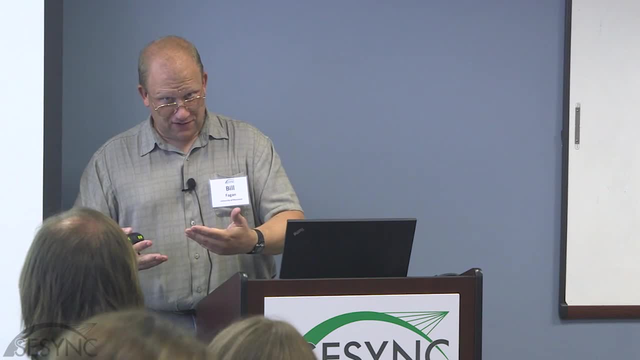 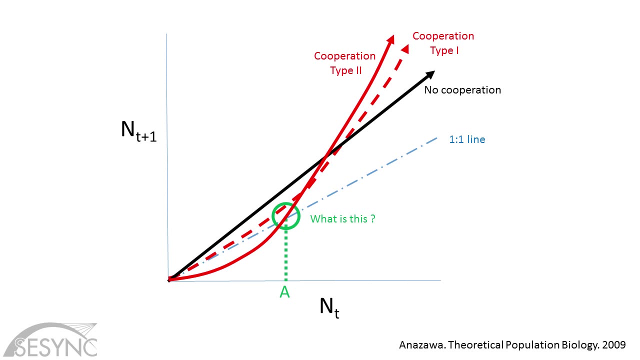 is the population unable to replace itself, And so we can think about this crossing point as a key threshold, Because below this population density we're down here in this region, this below this threshold A, and if we have a population size below this and we go up, 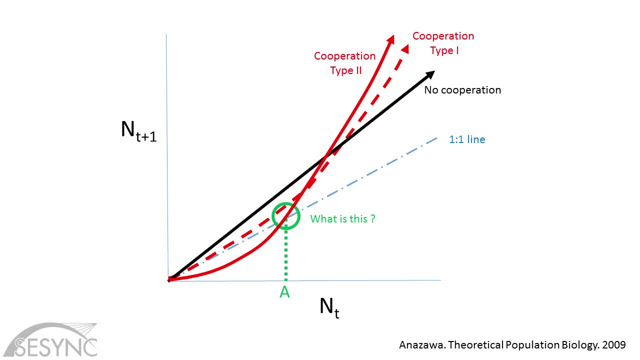 we hit the red curve and we go over to the left. on this axis our population is going to be smaller than where we started, So these differences are going to be important. Different kinds of curves have different names. in ecology They're called alley effects. 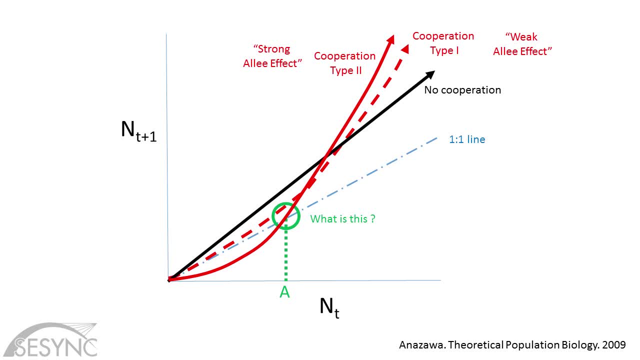 And people differentiate them in terms of a weak alley effect in which the red curve never crosses that one-to-one line, or a strong alley effect in which the red curve does cross and you have that strong thresholding effect that can cause a population to decline. 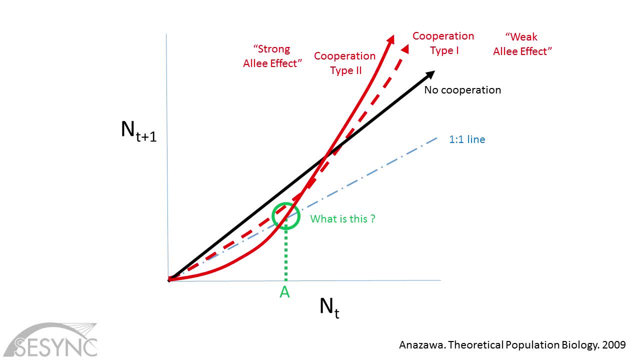 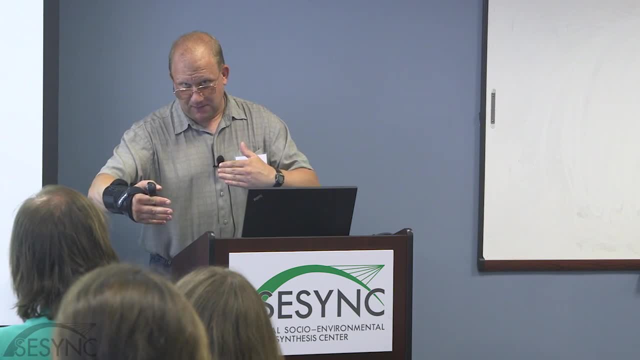 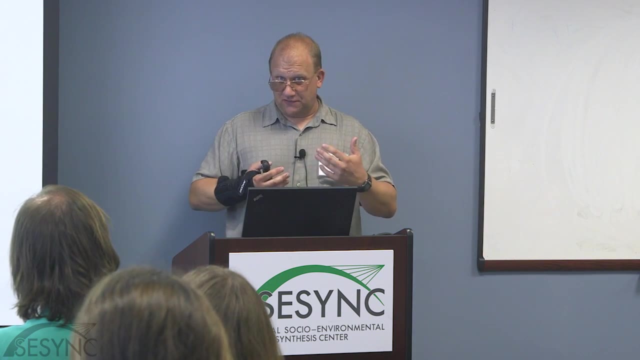 if the population is for some reason pushed below that threshold, A Cooperation among individuals has a bigger than one-to-one benefit. Okay, And so here are some examples of this kind of an effect. The ecologists call it an alley effect. It has other terms in other fields. 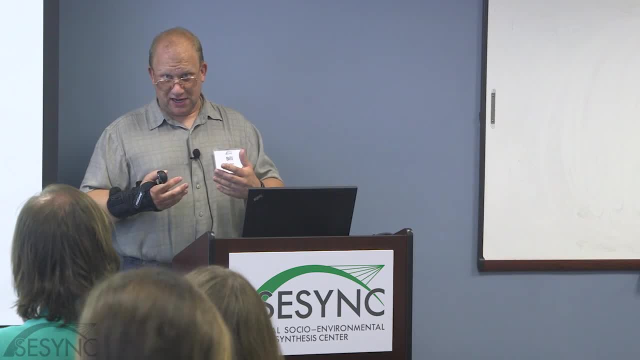 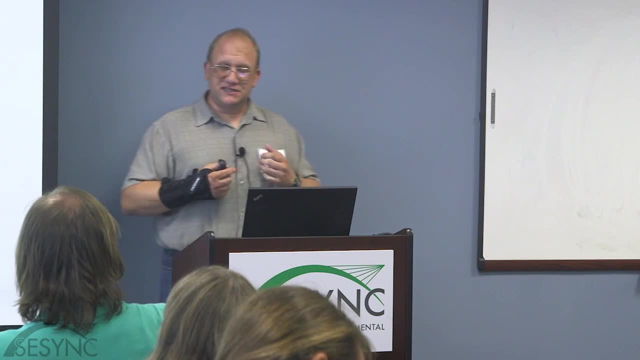 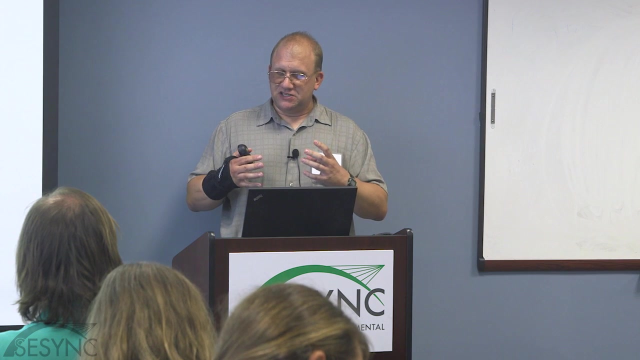 Autocatalysis is one, Cooperation is one in social sciences, But the idea is that there's a critical threshold where the dynamics change. This is sometimes called positive density dependence- Okay, And the idea is that interactions among individuals of some species are more. 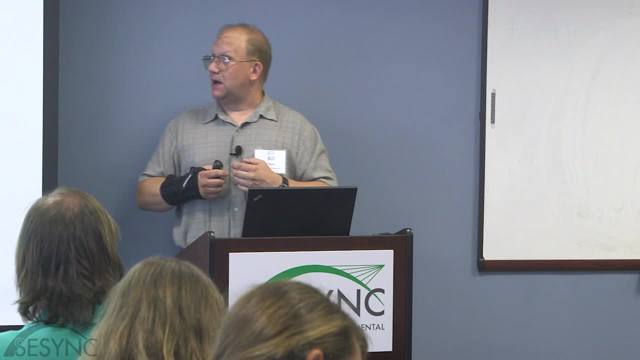 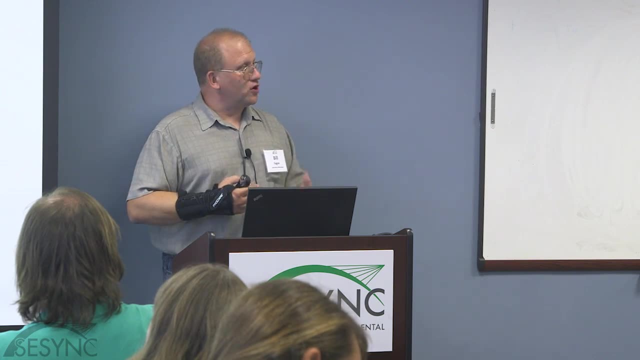 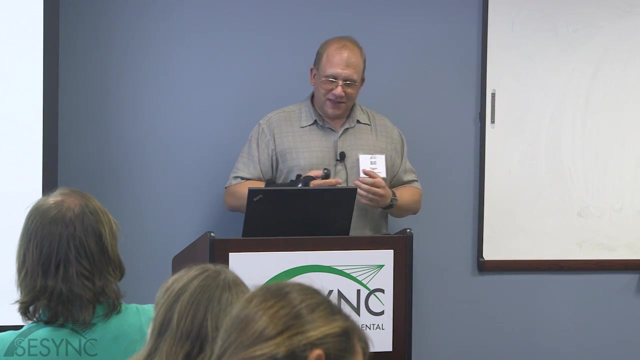 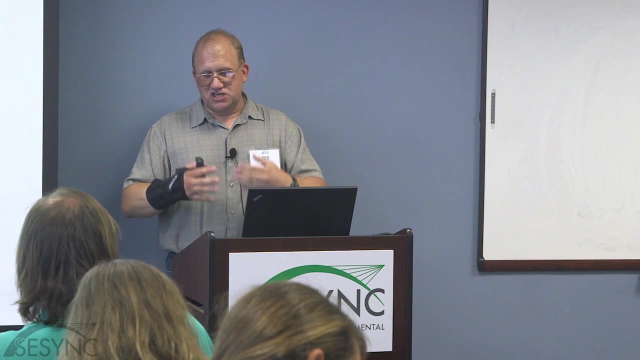 than additive in their advantage To the further growth of that population. This kind of super-additivity is applicable at the scale of organisms or cells, molecules and I would argue even groups of people or cultures. The idea is that there is a beneficial consequence of interacting together that leads 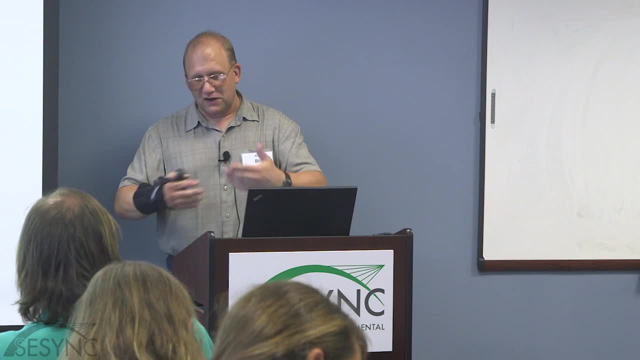 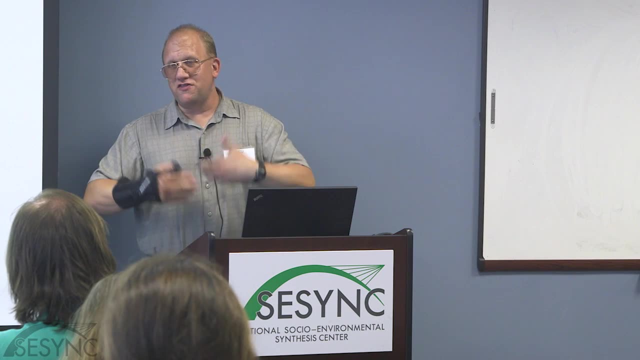 to a more than linear increase in population or in whatever your metric is that you're focusing on. But because this is population ecology, we're going to talk about this in a little bit. The metric is population size And it's this more than linear benefit from the interaction. 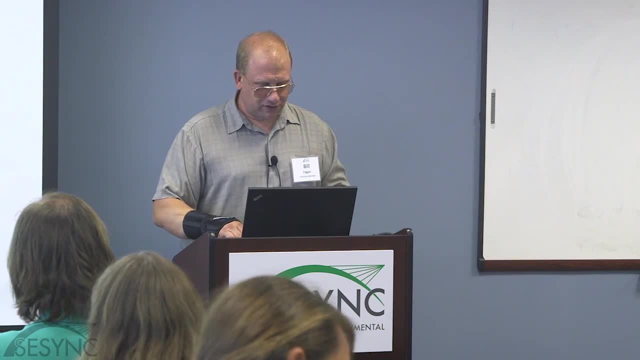 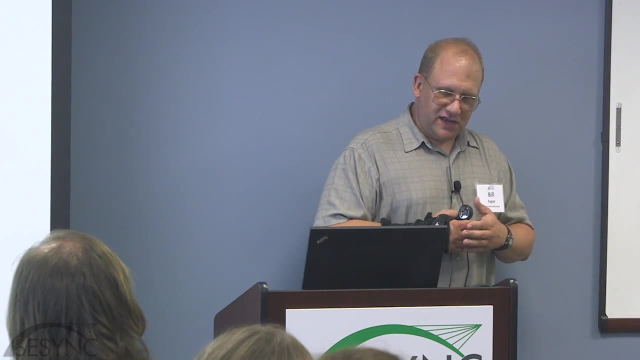 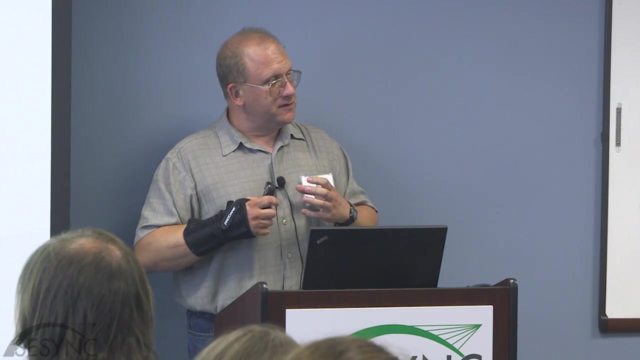 that leads to this kind of curve that I showed in the previous slide. Ecological mechanisms that can lead to this kind of an effect are really widespread in the world. You can have mutual shading by plants, So if you're in a harsh desert environment, 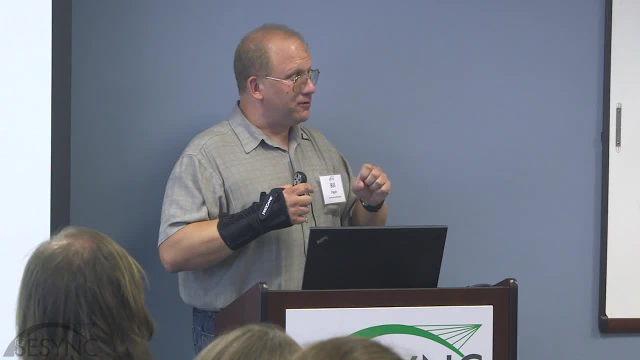 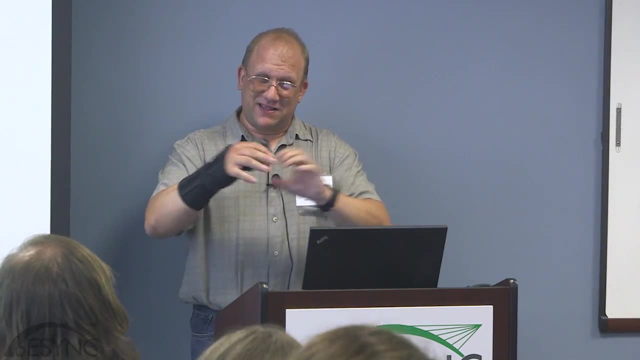 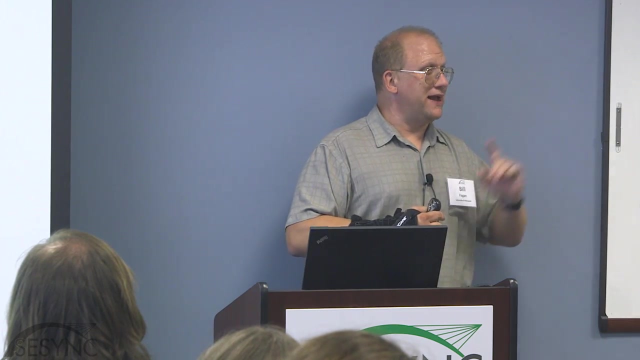 the idea that plants can provide some benefit to their neighbor to help reduce water loss. the more plants you have in an area, the more benefit that there might be from that spatial positioning. that would not be possible for a plant that's all by itself in the direct sunlight. So there's a benefit from having the plants interacting with one another to provide that benefit. You can also think of this happening in mutual defense by groups of animals, A good example that I like to use because you can sort of picture it in your mind. 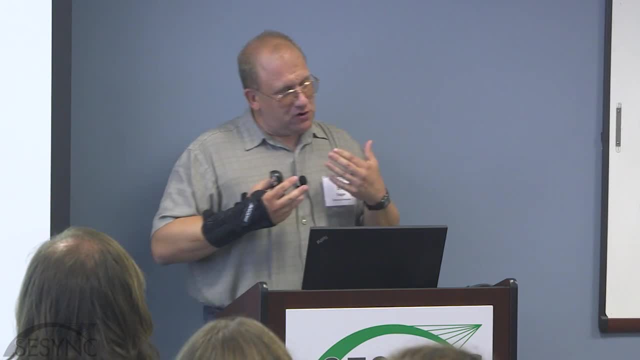 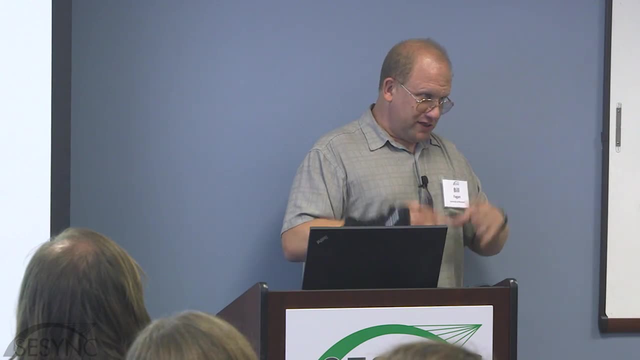 is a herd of musk oxen If you're in the far north, the herd of musk oxen. the strategy for defending themselves from wolves is to form a circle, with their fierce horns pointing out, And they put the little calves in the middle. 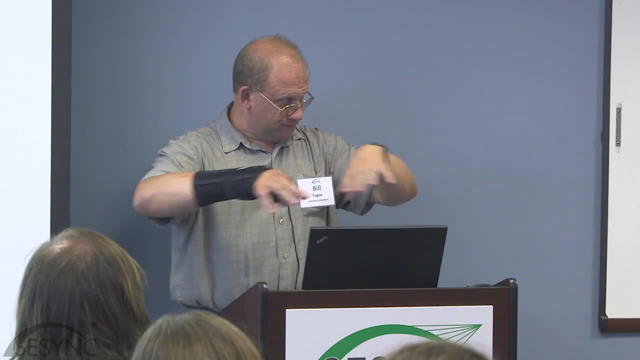 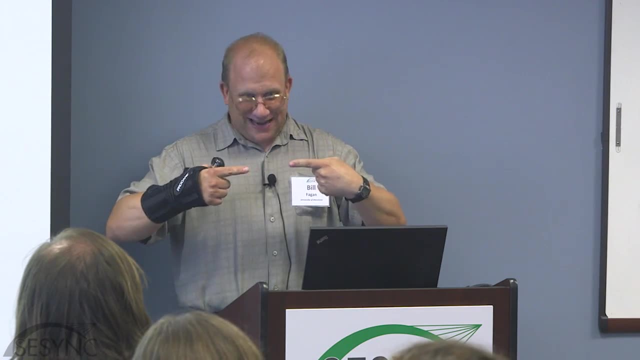 If you have enough musk oxen, you can form a complete circle And you can protect your calves. If you have two musk oxen, you put them back to back and you can get at them, but from the side. 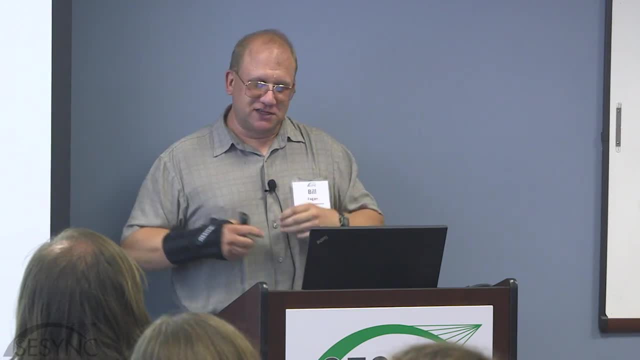 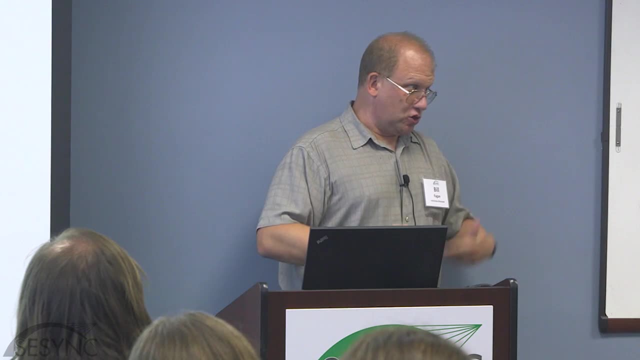 So it becomes an issue of spatial reinforcement. that's possible by virtue of having more than enough individuals to cooperate in some way. The same thing could also be said about the wolves right, Because they need to have enough individuals working together to bring down the musk oxen. 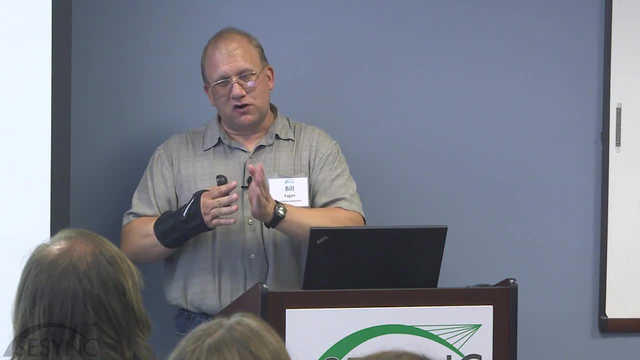 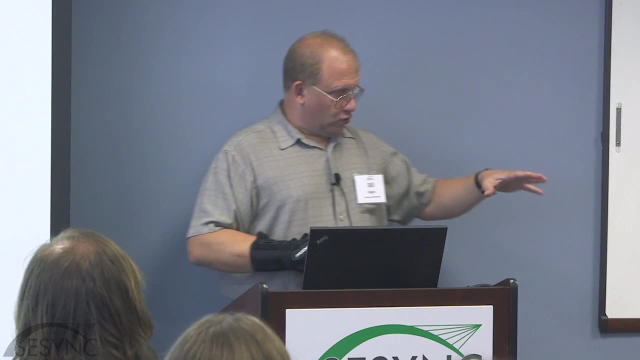 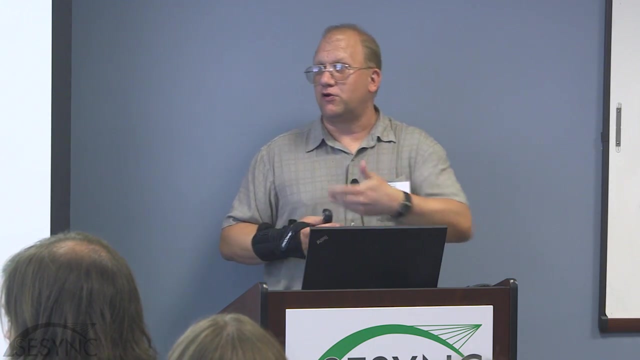 But the issue is cooperation and that you need some kind of a critical threshold in order to get that very different kind of super additive response. In the molecular world you have the same kind of uh process going on. You can have molecules that facilitate the production of more of their own kind. 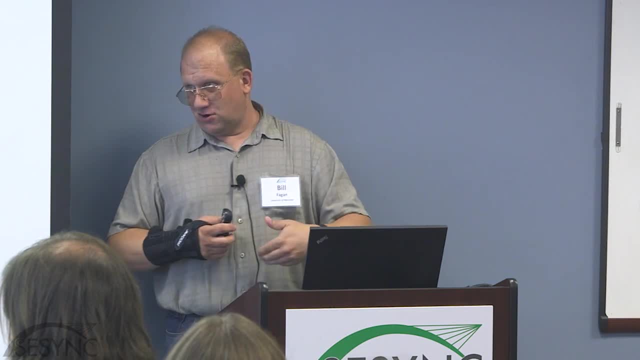 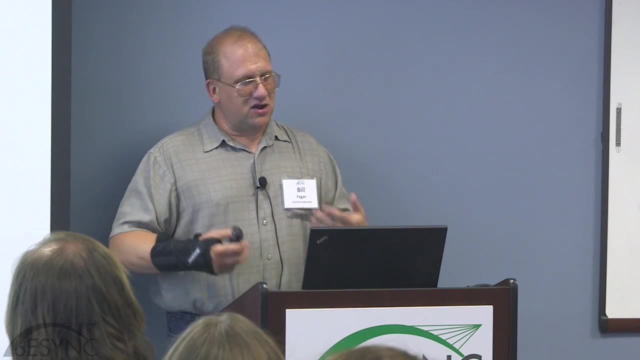 This is a situation, for example, where proteins can impact RNA synthesis that then influence the rate of more proteins at which they're produced. This is physically it's auto-catalysis, And so mathematically we get that non-linearity. 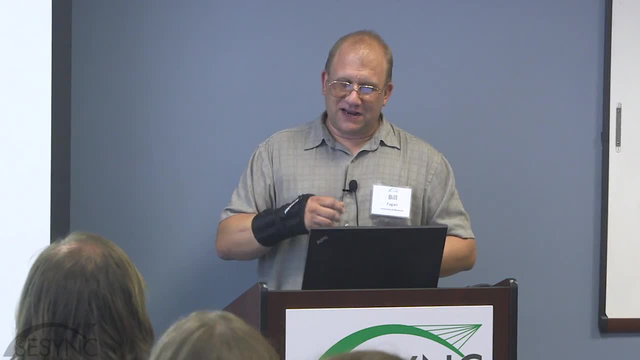 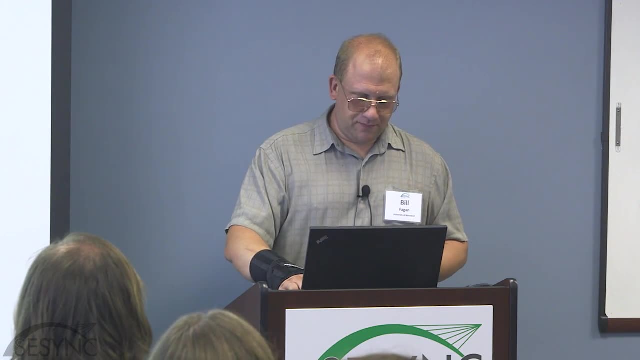 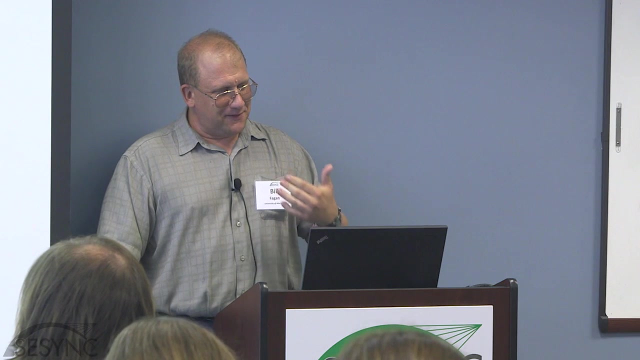 We get a departure from that straight-line curve that comes about by virtue of individuals interacting with one another, uh, in a effectively cooperative way. Okay, So the third law that Berryman introduced is the idea that coop- competition among individuals can occur. 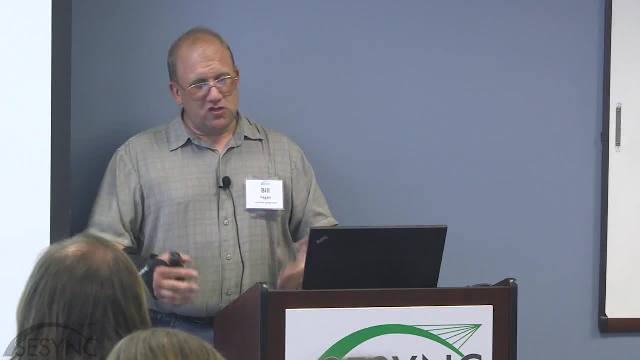 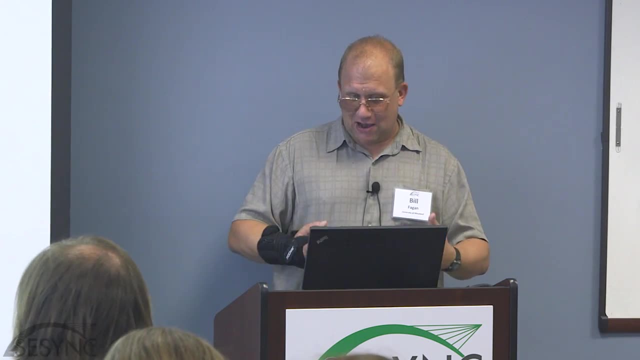 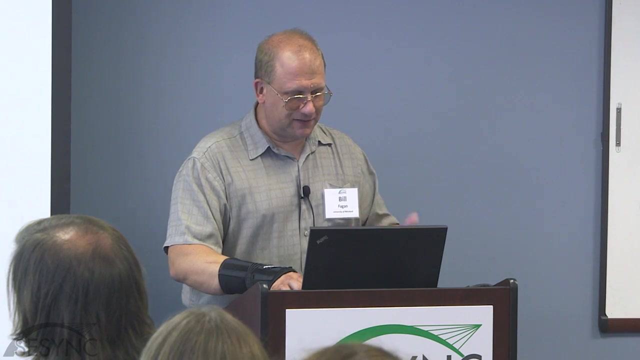 and that, in other words, there's too much of a good thing. So, even though cooperation might be beneficial under some circumstances, eventually things might get too complicated, too crowded, and that competition among individuals, um Can can have negative impacts instead of the simply positive ones. 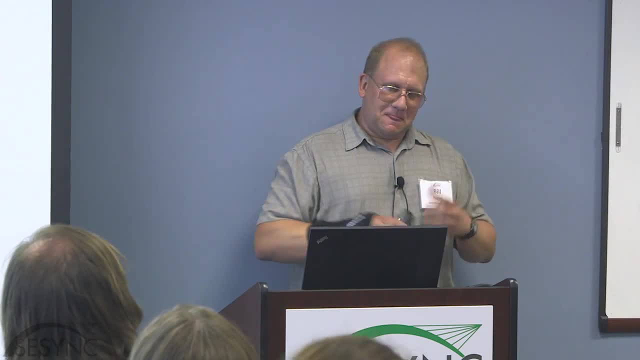 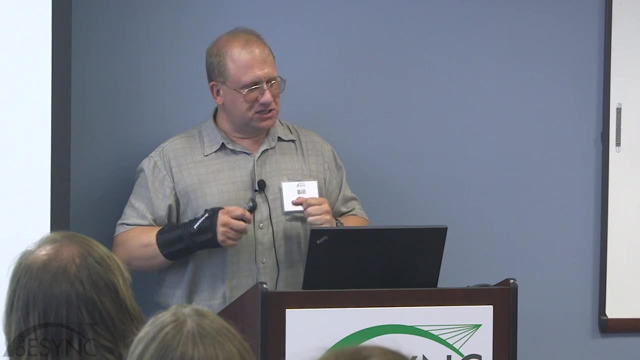 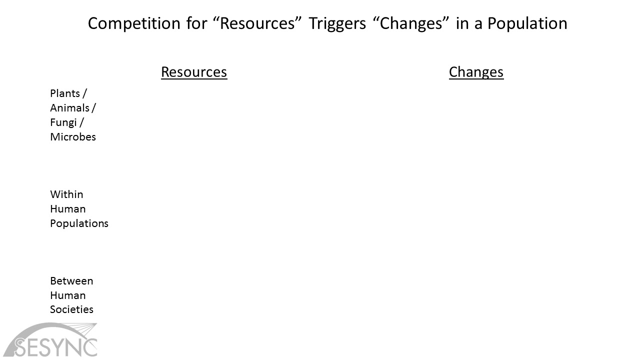 Okay, and so the idea here is that in in very broad, very general terms, competition for resources Triggers some change in a population. So let's think about that in different contexts. So let's think about whether we're in the first top row of examples. 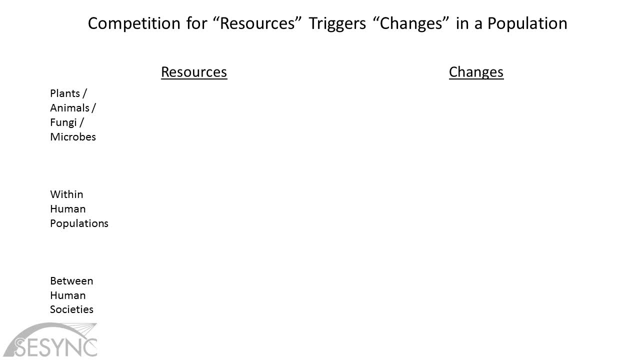 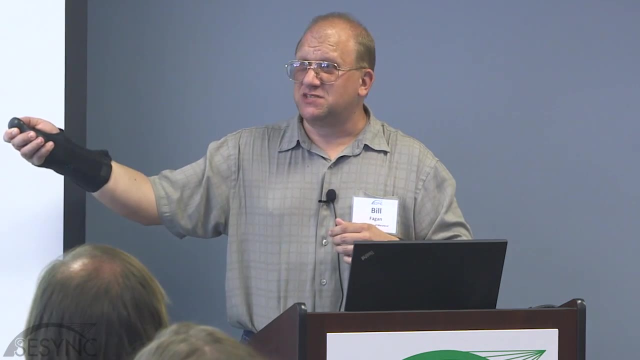 We've got ecological species, Okay. Down here in the middle we have what's going on within a human population, and then at the bottom I'm going to talk about between human societies, Okay, and in each case we can think about what the resources might be and what kind of changes might take place as 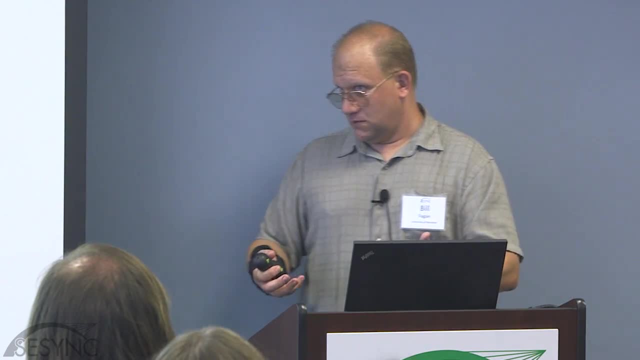 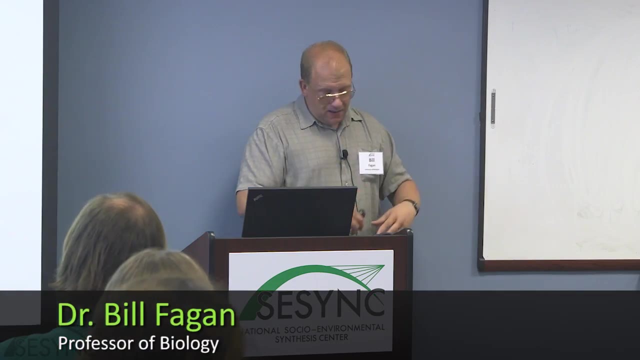 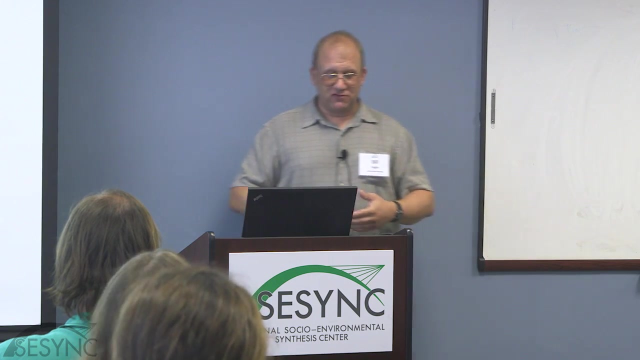 those resources become competed for. Okay, so let's try to fill this in a little bit. So there's a fixed amount of light that's irradiating the area and that There may not be enough for all individuals to get enough light to grow. Okay, and so if the resource is light, They're competing for light. a Change that might manifest in that case would be an increased rate of mortality, Because you've got more seedlings dying because they can't get the night late that they need to grow. Okay, How about in social systems? What happens if we have a human population? 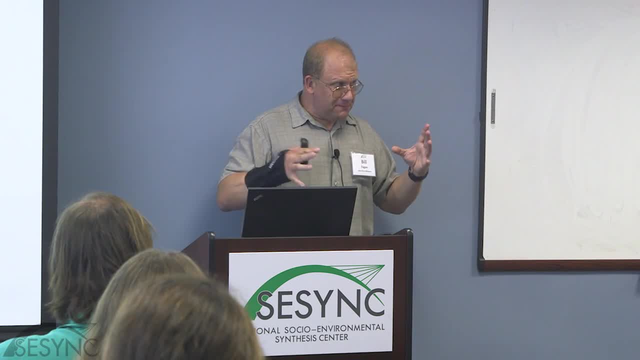 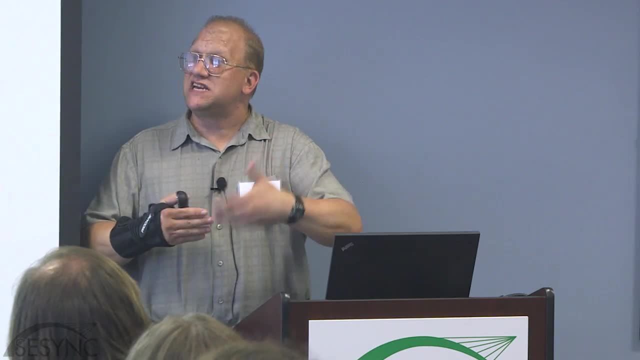 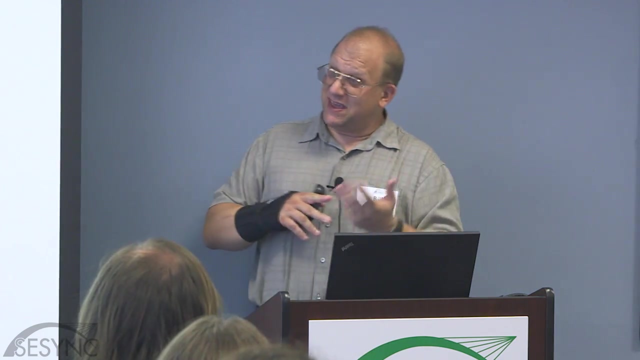 What resource might exist and what might happen when people within a population Start competing for that resource. What kind of change might we expect? This is the key thing is that there's many different responses to it. to a given Competition for a resource- the example you gave- people might leave the area. 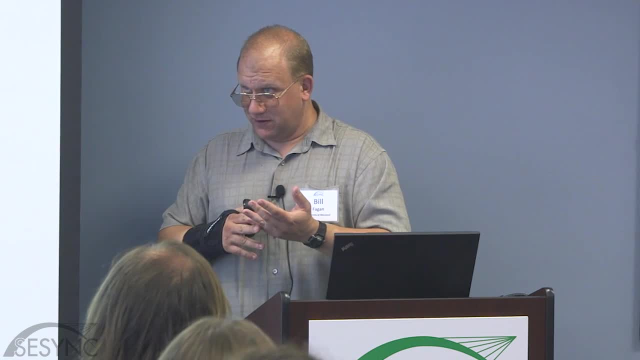 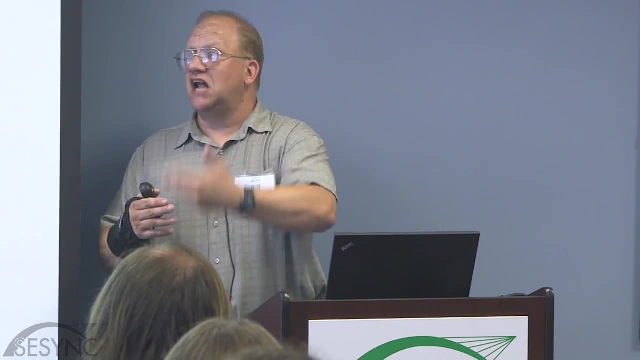 People might, you know, have some kind of hostility with each other. they might engage in some kind of treaty to better share the resource. but there's going to be a consequence because the resource itself is limiting. it's going to trigger some change when the density gets too high. the 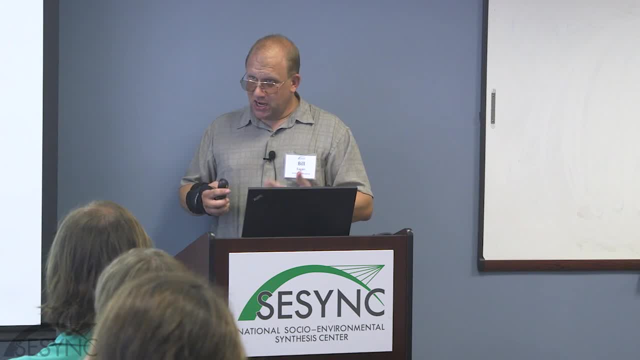 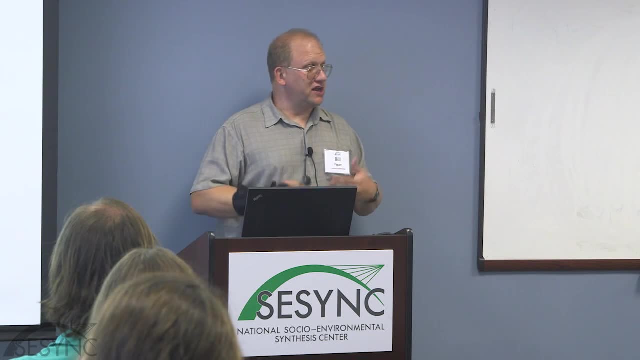 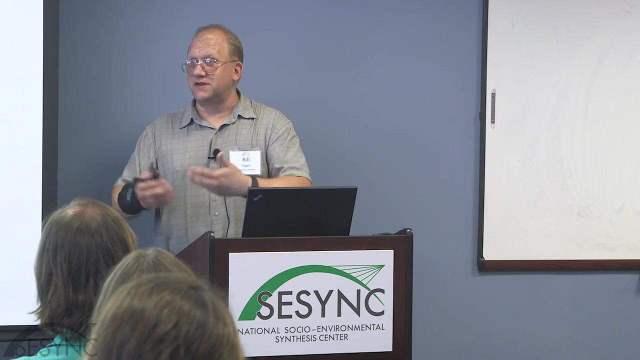 Pitch, then, that I would like to make is that this kind of conceptualization is one way in which the mathematics and the Graphical approaches that ecologists have developed to study competition as a force within Wildlife or plant species can carry over and help mathematize. 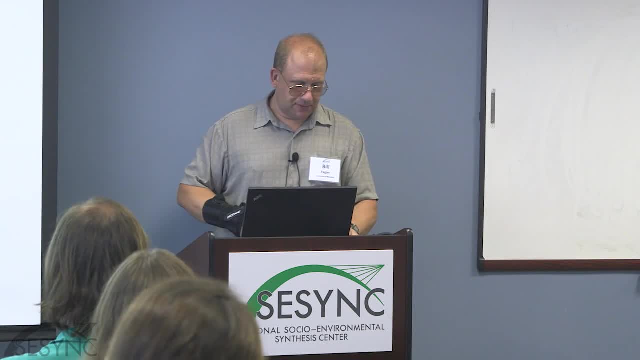 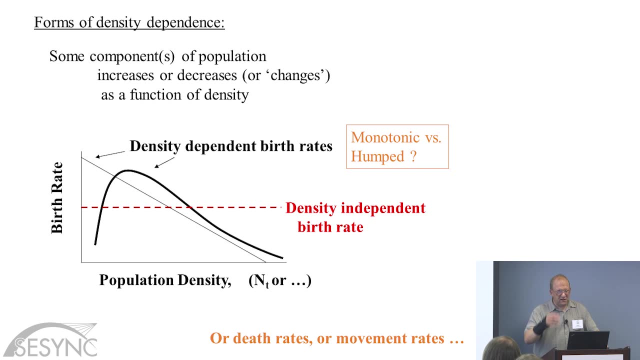 Problems. in social sciences It's a very similar concept and the tools are already well developed. We can talk about transference. Okay. so some example then of Density-independence in the ecological setting, Some component of a population is going to increase or decrease or change in some way as a function of density. 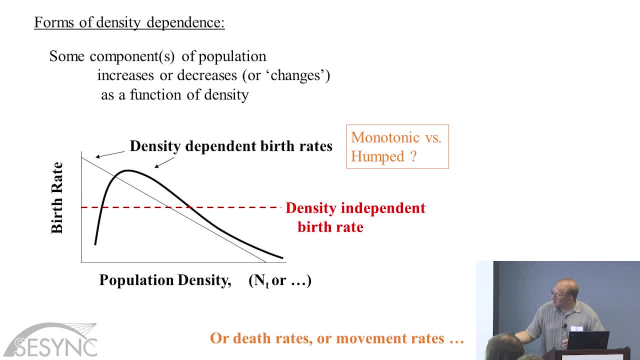 So this plot here shows what this might look like. We might have our population density again, That's our N, Something that is density-independent, does not change as we go from very low to very high densities. But in these cases here in the black curves have a situation where some parameter, in this case birth rate, shows a functional dependence. 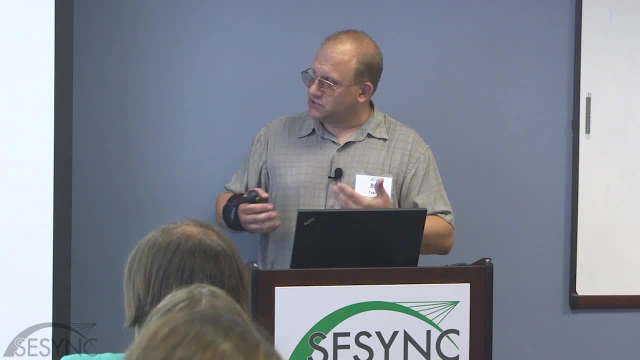 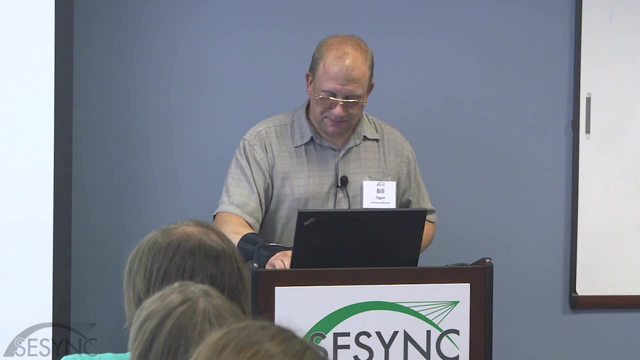 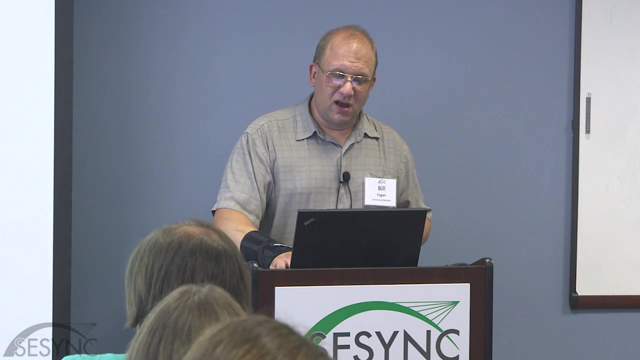 on population density And that's kind of our visual characterization of what we mean by density dependent versus density independent. And of course, what we're talking about need not be birth rate, it could be movement or death or some other measure of interest. So, going back to 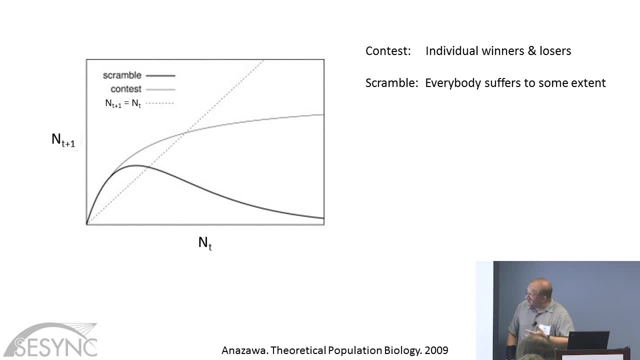 Anazawa's plots. here's an example of how this might look on our plot of population size at time, t versus t plus one, And here's our one-to-one line And you can see that there's these two different kinds of shapes that are possible And ecologists have given these different kinds. 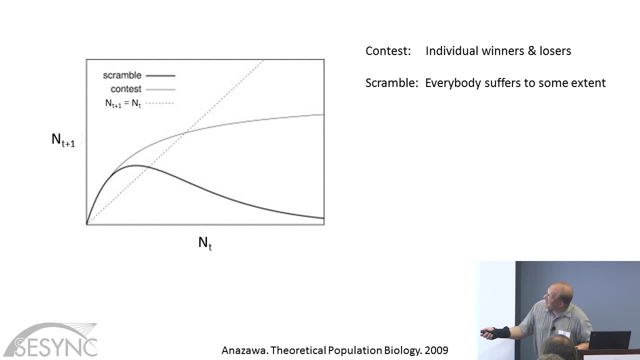 of competition names And the curve here it shows this big hump and then comes crashing down- is called scramble competition And this other one up here is called contest competition. The idea is that these represent different kinds of interactions, different outcomes to the way the competition plays out In contest. 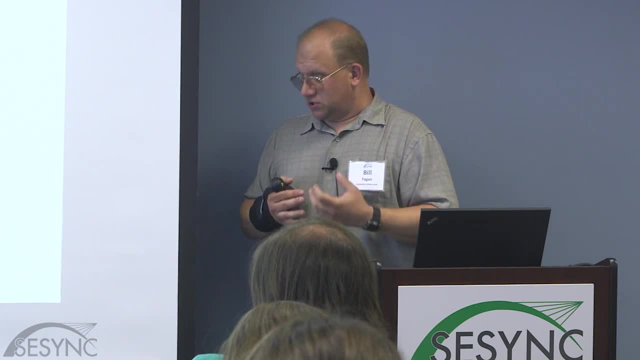 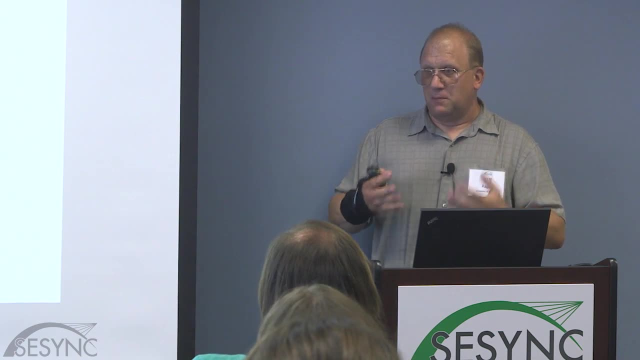 competition. the key issue is that there are individual winners and losers, So you can think of a resource that is discrete in some way so that it could, for example, be a occupied. It might be in the case of some cavity-nesting woodpecker. the number of cavities 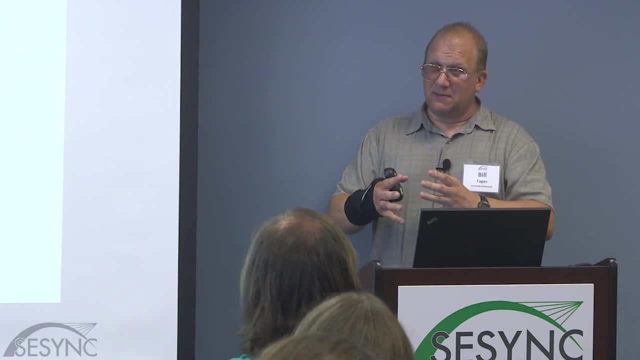 in the trees that one pair of birds gets to occupy it, And if you don't have enough cavities but you have more birds, then the ones that are not in that cavity don't get to reproduce. We might think in human systems it could be wells or some other kind of limiting resource that. could provide a structural spatial organizing principle. The contrast is in scramble competition, where everybody suffers to some extent. It's not like there's a discrete resource which could be obtained and held onto, but by virtue of competing for that limiting resource, nobody. 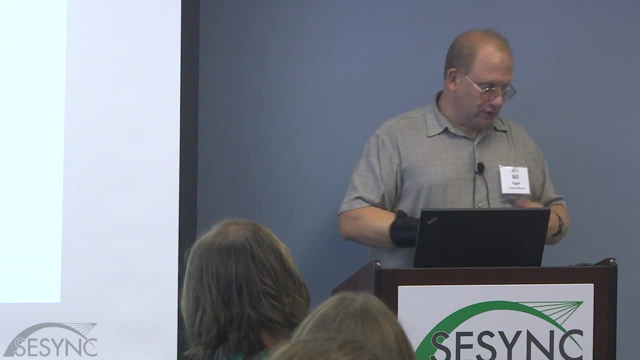 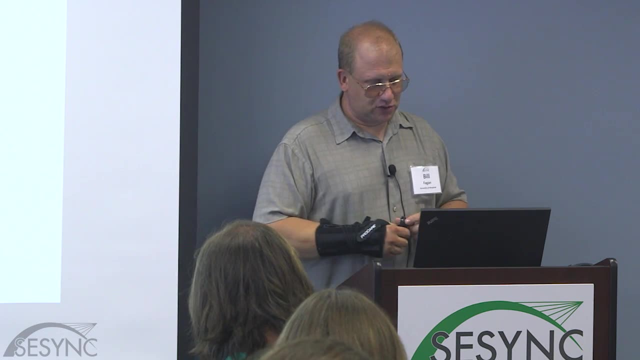 gets enough and as a result, everybody's output, whether it's reproduction or lifetime or some other kinds of measure, suffers as a result of that competition for the resource. Now we can think of the same kind of plot Here. it is putting the two things together. 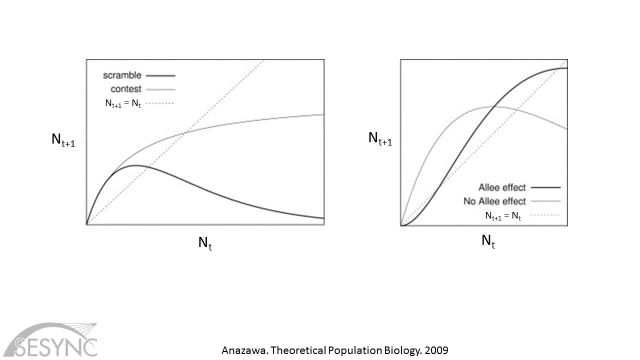 You've got an alley effect or no alley effect Together with the two different kinds of competition and you can see that you can have both positive density dependence- down here at low densities- and negative density dependence- up here at high densities- taking place Graphically. we can think of the response around this. 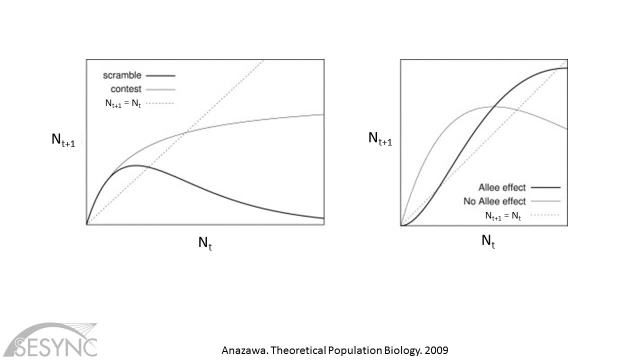 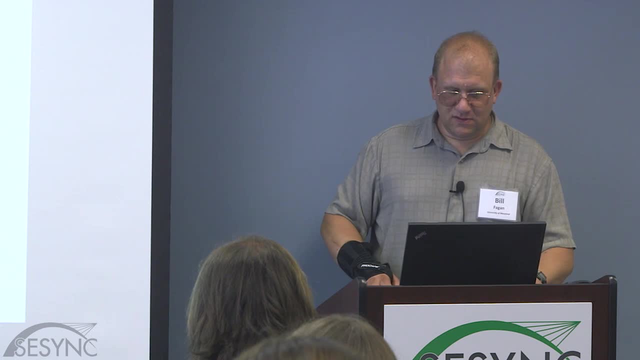 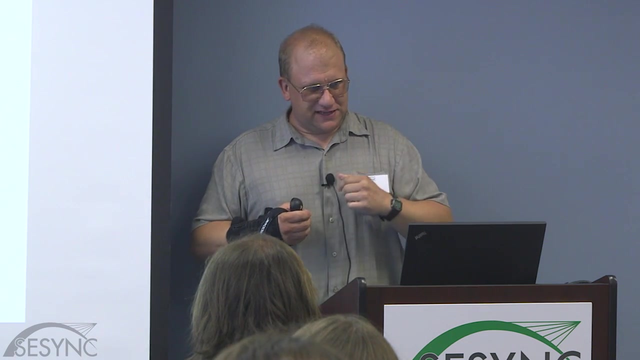 one-to-one curve as a guide for helping to understand how changes in density translate into these different impacts on the population. So, mathematically, let's think about this. switch back Again. if we want to talk about mathematics of density dependence, it's easiest to see: 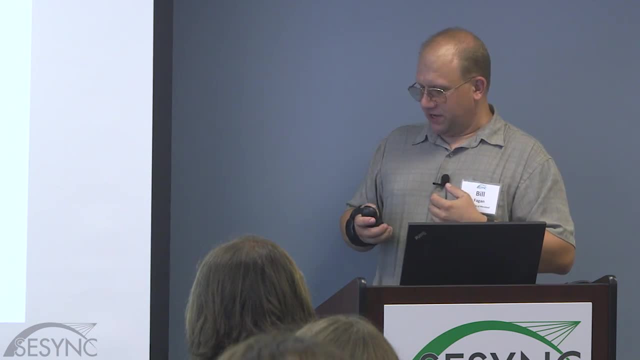 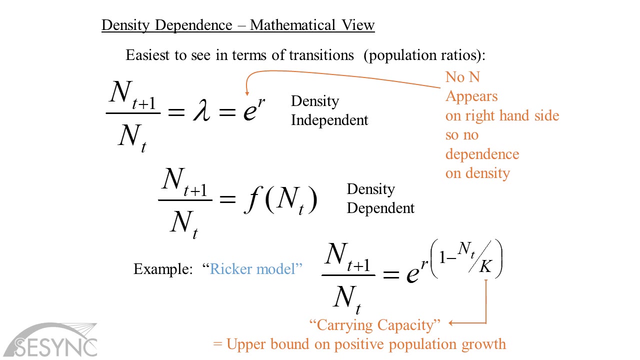 if we focus on the transitions, so population ratios. So in this case we have a ratio of population size of t plus 1 relative to p and that is our population multiplier lambda. Sometimes it's written e to the r. This is a density-independent framework. It's density-independent. 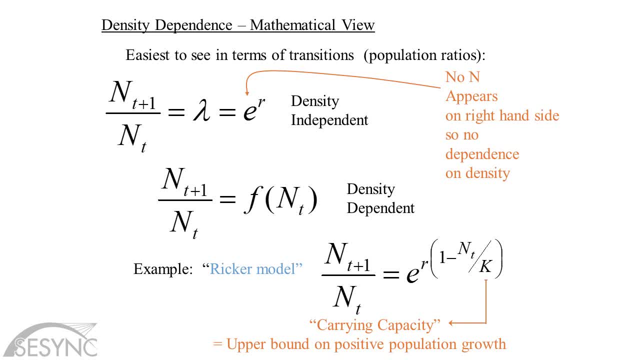 in a mathematics way, because we can see that the density n does not appear on the right hand side. So linguistically it's density-independent, because the population growth does not depend in any way on density. Down here is a form in which there is density dependence, because 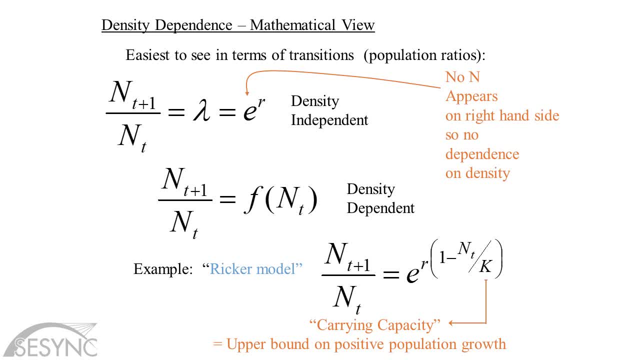 there is some function of population density on the right hand side of that ratio. An example in fisheries literature is the Ricker model. This is the Ricker model for population growth of a fishery stock. It introduces this common concept called a carrying capacity. The parameter now is k And the ratio of change between 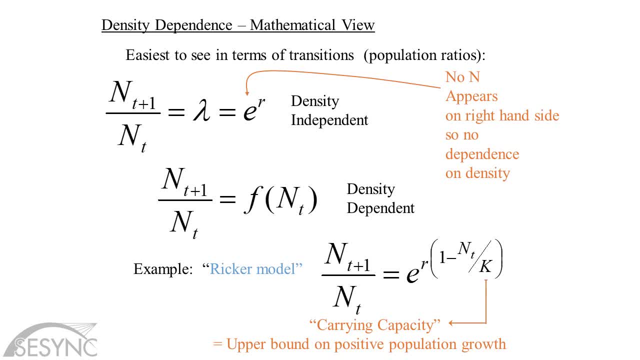 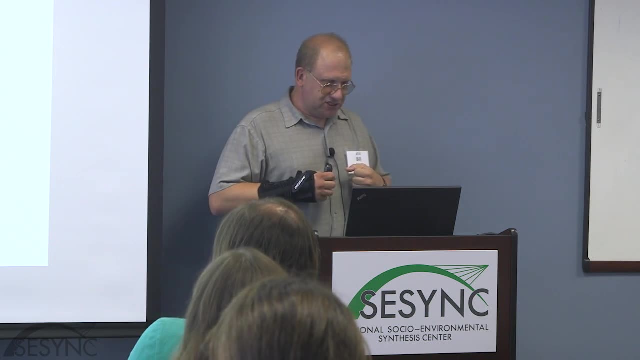 time steps is governed not by e to the r, but by e to the r, with this term in parenthesis- which governs the limiting effect of increasing density on the population. There's a huge cottage industry that is interested in the mathematics of population dynamics in part. 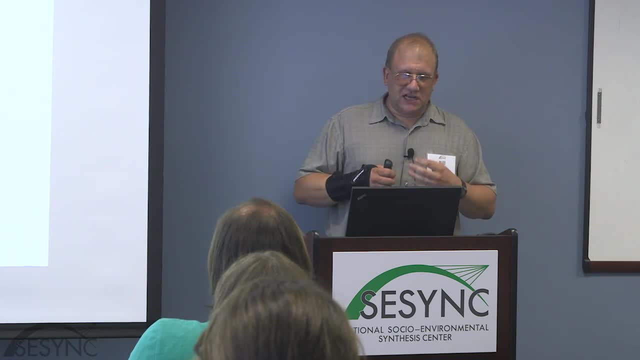 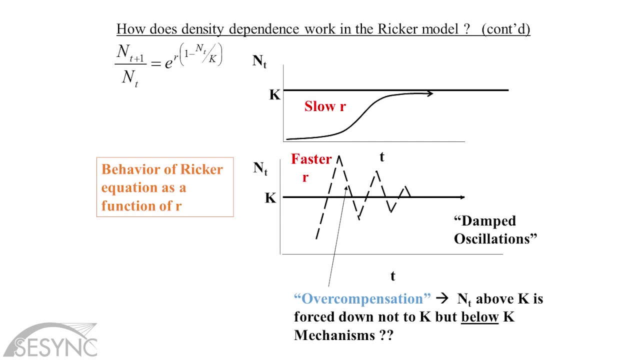 because of the interesting behavior that these kinds of equations can produce. So, for example, if we take that Ricker equation and we play with the value of r and we'll just call it slow and fast, r, small and large, If we have a small value of r, then the population 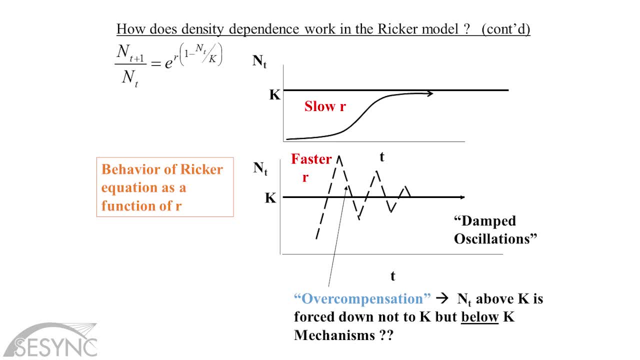 size as population size. n- as a function of time, t- note that I've changed the axes now, so everything now is playing out as a function of t, time. then if you have a low value of r, the population in this model will increase. 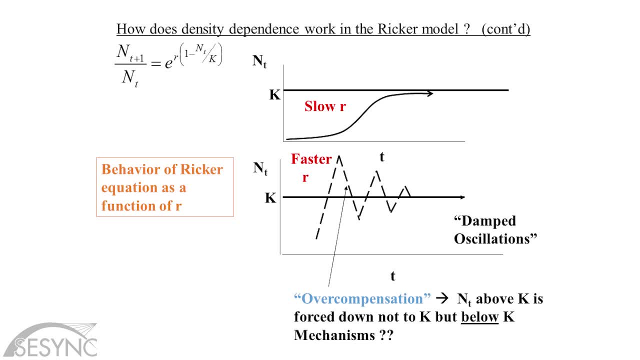 So if you have a low value of r, the population in this model will increase. and if you have a high value of r, then the population will increase, Increase, will increase. but wait until you have a low value of r. So you push nagyonije más duido. 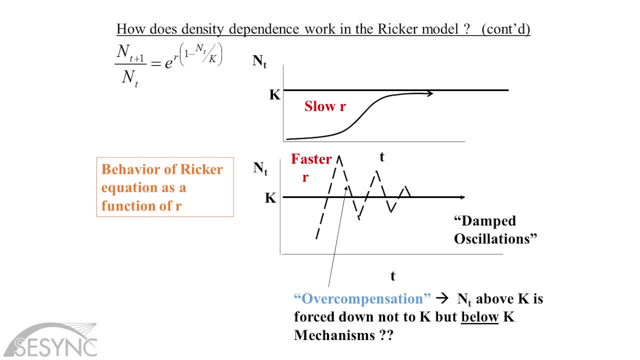 raise to a very different kind of result. In this case, it leads to what are called damped oscillations. The population does not slowly and gradually approach r or approach k, rather, but it bounces around as it converges on that value. This is this compensatory. 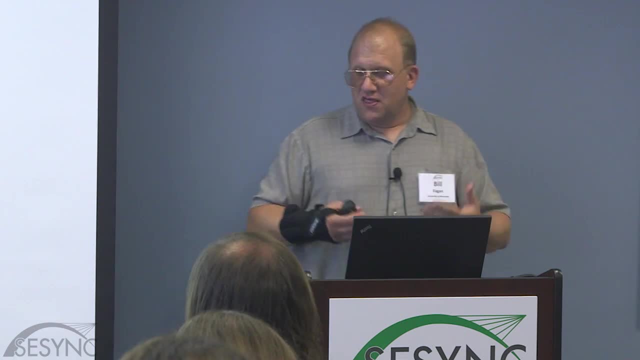 over compensatory dynamics. that arises because the fast growth rate of the population pushes population size so far above K that everything collapses down far below carrying capacity for the next time step. Okay, get that. The population size is pushed up by the fast growth rate. 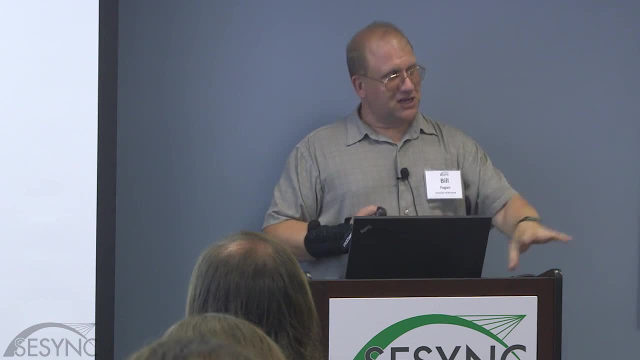 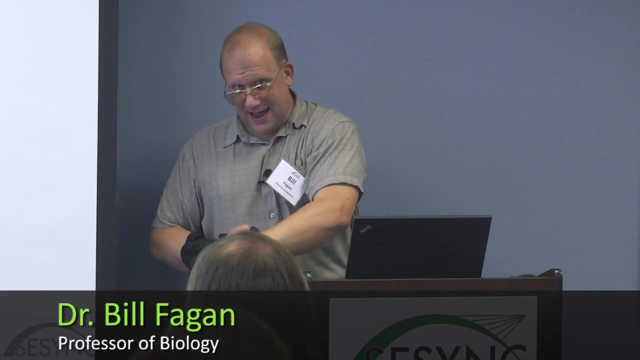 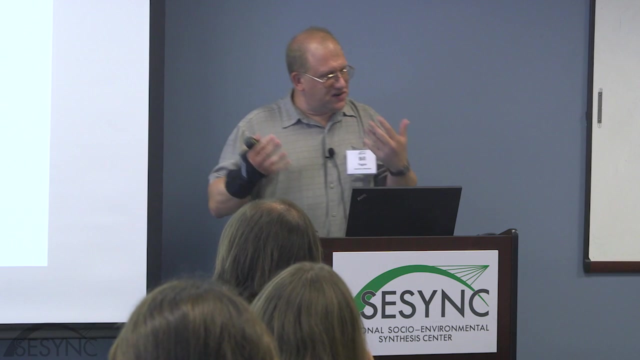 Density dependence kicks in and the population collapses down far below K. So what are some mechanisms that can give rise to this kind of up and then down? The idea is that the parameters of our model give very different, qualitatively different behavior. 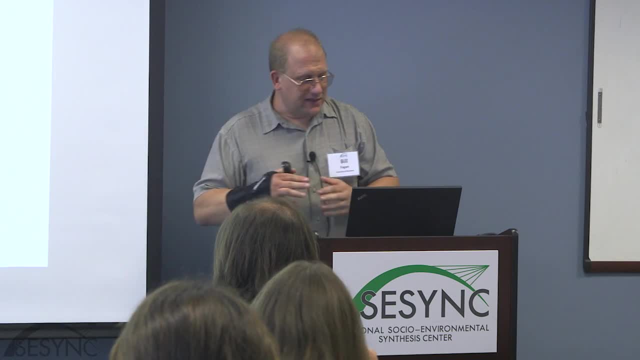 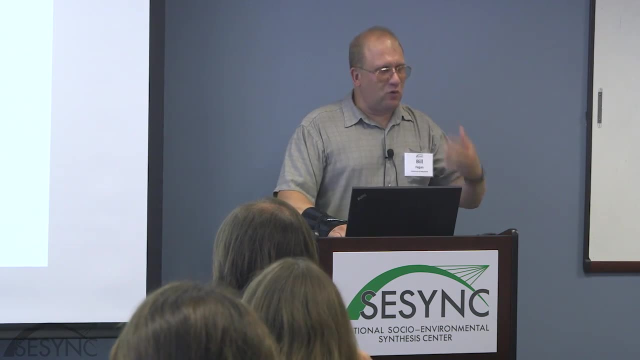 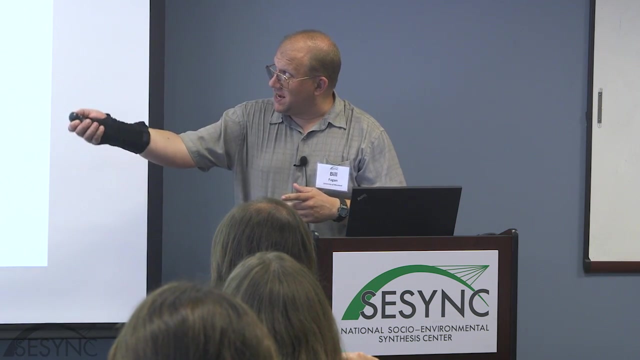 and that it actually gets more complicated than this, But the idea is that that single equation can give rise to very different dynamics. If we were watching the population respond, we could see very different scenarios, but the underlying dynamics would be exactly the same. 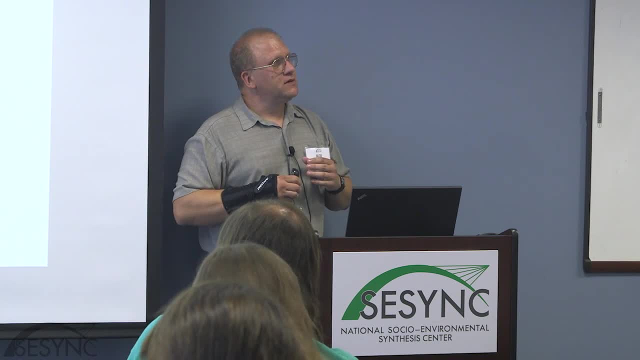 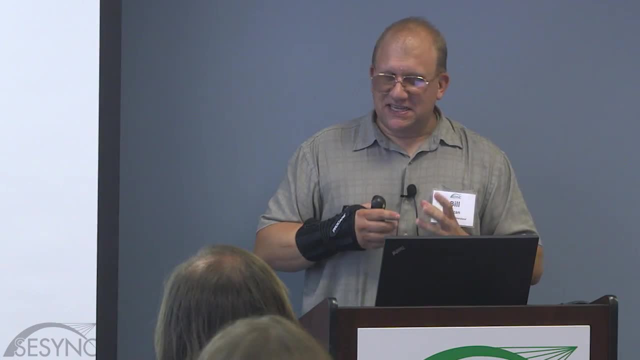 So let's think about this in a situation that kind of steps forward a little bit to a more complex situation. The idea is that the strength of density dependence can itself be a tunable parameter. So in other words, there is another kind of model. 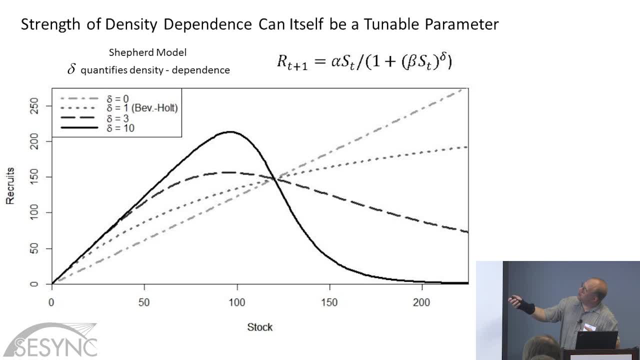 which is used in the fisheries literature, where we have another parameter called delta, and parameter delta governs how strongly the population responds to increases in density. We can have these different kinds of responses taking place as we change the value of delta. So in gray dots here we have no density dependence. 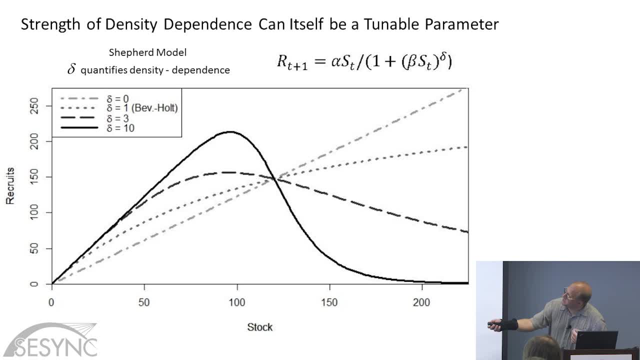 delta equals zero. We start setting other values: delta equals one, delta equals three, delta equals ten- and we get very different shaped curves on our relationship between the breeding stock- in this case of fishes- and the number of recruits that are produced. 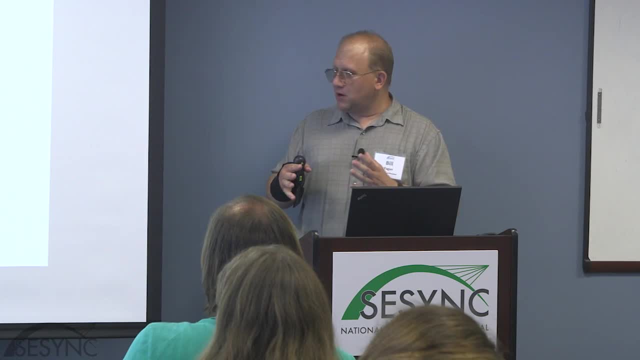 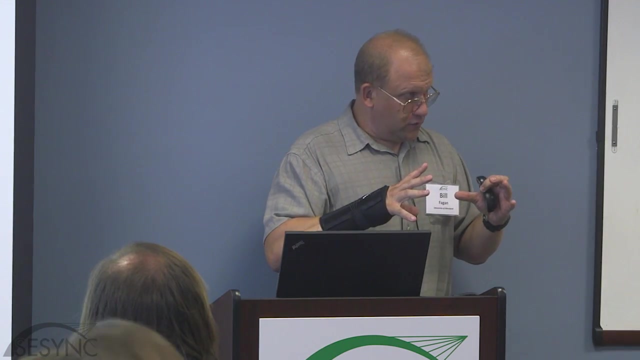 from that breeding stock. The same equation, with density dependence now being a tunable parameter, gives us different ways in which the population might respond as the density changes. Let's think about this as a single framework that we can use to study a whole host of different species. 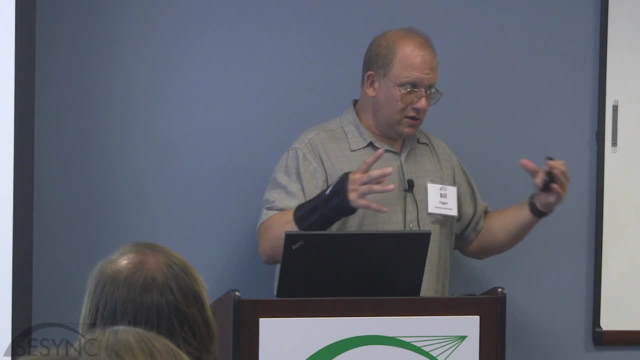 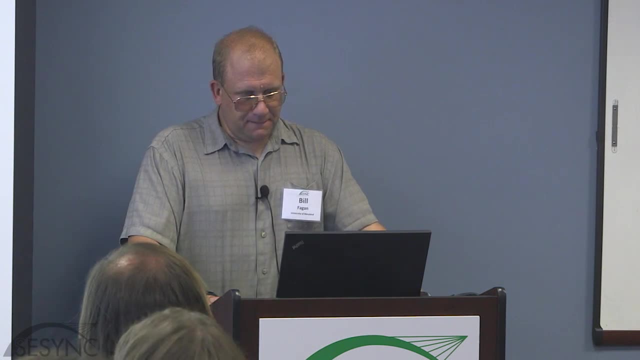 that are going to differ from one another in, let's say, their life history traits. Okay, And life history traits can include things like the number of eggs deposited, how that changes as a function of body size, lifespan, the age at which they become reproductively active. 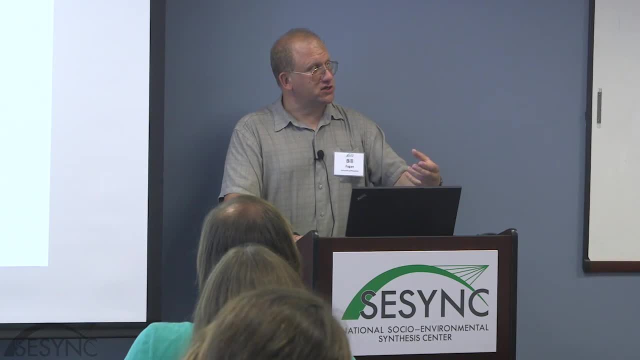 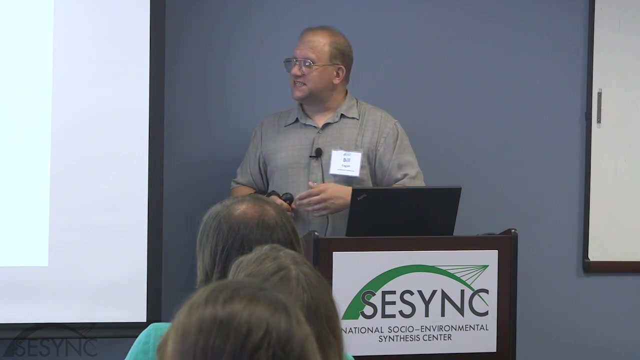 All of these things are traits which govern the rate of reproduction, which can vary from one species to the next, But we want to have a common framework for trying to pull all this stuff together and matching it with fisheries data. okay, The trouble is that it's notoriously difficult. 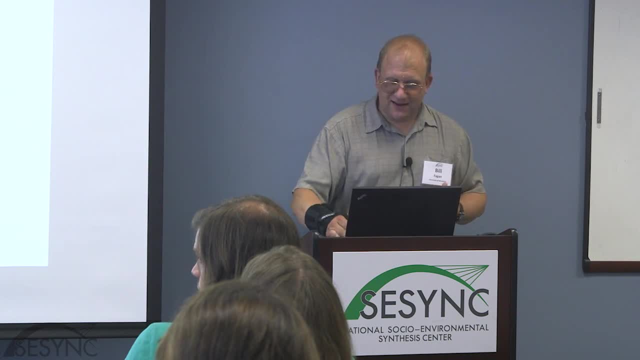 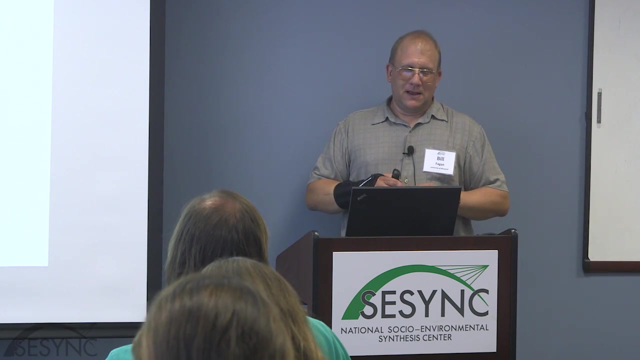 to estimate the strength of density dependence, Despite the fact that density dependence can give you all this kind of radically different behavior. it's critical to the underlying population dynamics, but actually estimating it is a real double of a problem. Why do you think that might be? 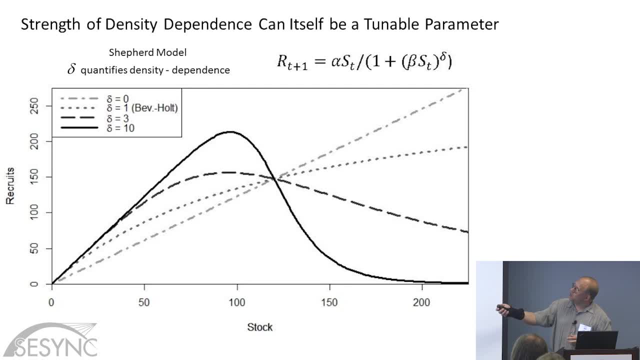 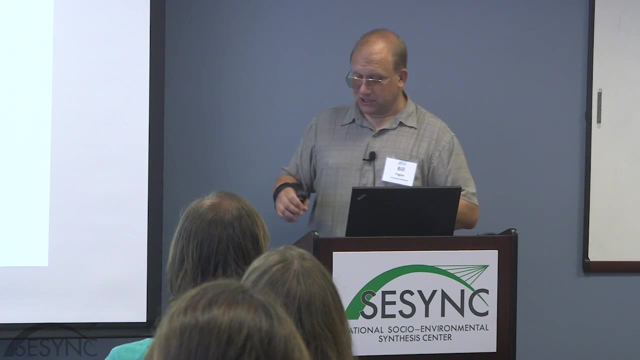 Why would this be hard? This is an equation for one population, okay, And these represent different curves when you choose different values of delta, So they could represent. you could have them represent one species. they could represent different species, different populations. 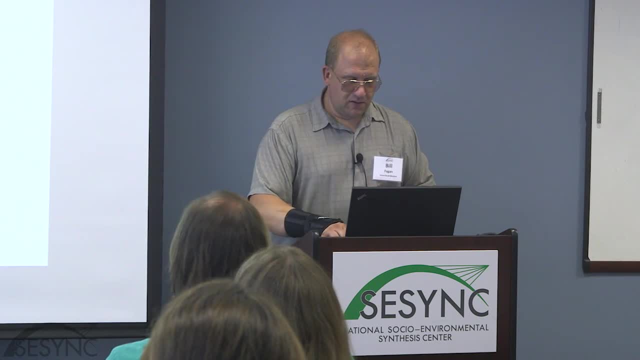 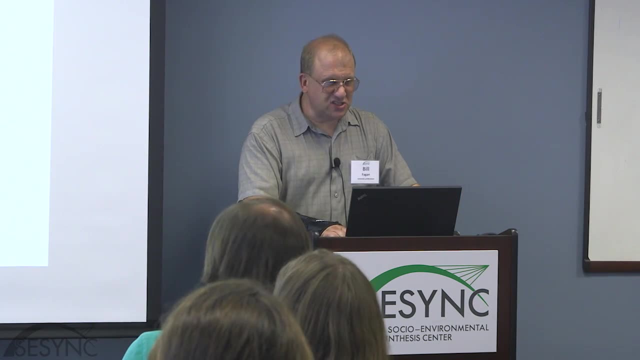 It's just showing the flexibility of that particular model. So why would it be difficult to estimate density dependence? It seems like a straightforward concept. So here's just a small list of things that are leading to the difficulty. So you've got the ability to estimate density dependence. 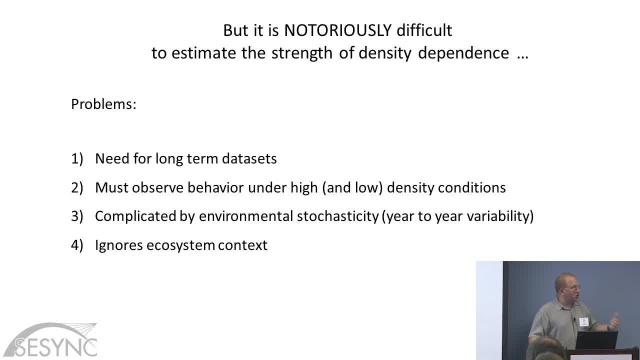 in real data sets that ecologists work with. First off, you need long-term data in order to make these kind of estimates. Because you've got, you might have a curve that has, you know, a complex shape to it and you have to try to estimate that. 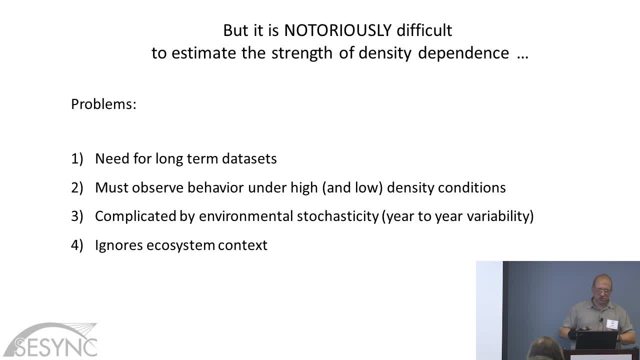 Well, that's a lot harder than trying to estimate a straight line. okay, So you need more data, And long-term data, especially if you're dealing with something that reproduces annually- is very difficult to come by, And by long-term we're talking 30,, 40,, 50 years. 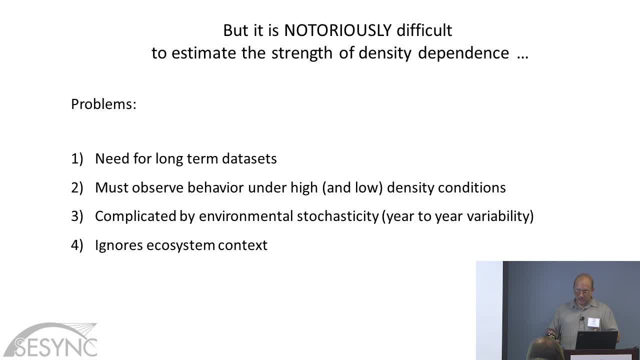 worth of data, And that's not something you can get during the span of a dissertation in most cases. The other complication is that you must be able to observe the population's response under conditions of both high and low density. This is a real challenge because in many cases, 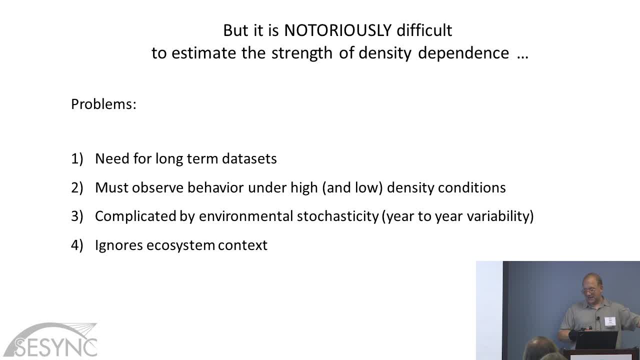 we don't want the population to go down to low density, Because bad things happen when that does, like fisheries crash, And so knowing the response under low density might be particularly difficult, And we want to try to avoid that, even though knowing that information would be helpful to us. You brought up the idea that you can have year-to-year variability. Ecologists that are doing the modeling call that stochasticity, that there's some kind of outside forcing factor which is going to add complications to our dynamics. It could, for example, have to do with the timing. 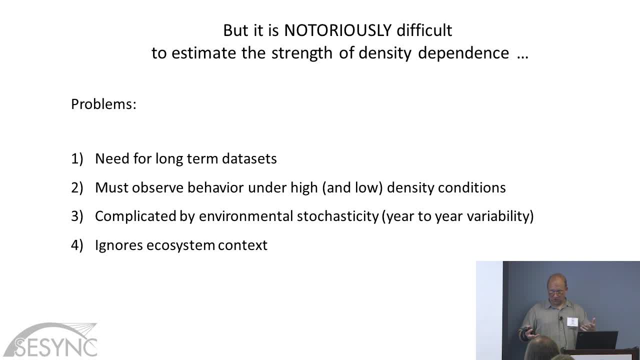 of an algal bloom relative to the time. So that's a big challenge And so you know we're trying to figure out how to do that And we can look at different ways that we can look at the timing relative to the timing of the larvae of the fish being released. 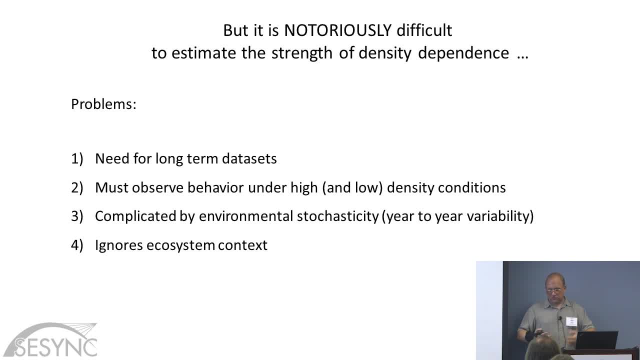 If those things are mismatched, you can have a very bad year for recruitment, But the next year the timing could be spot on and you get a huge boom year in terms of the recruitment of the larvae to a larger size fish. And the other point that you brought up is that this kind 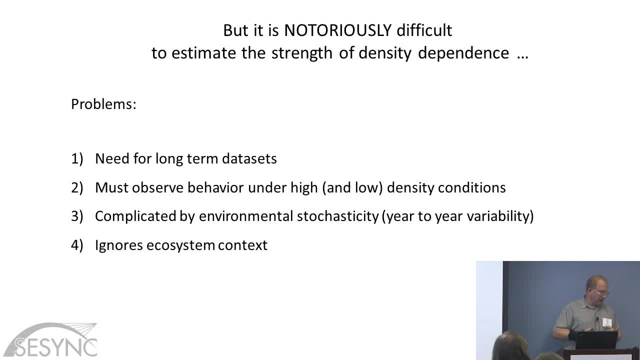 of approach totally ignores the ecosystem context. Okay, We're talking in the model. we just have a single population, It's just considered in isolation, We don't have it anything going on about its resources, the nutrients, the meteorological conditions, that. 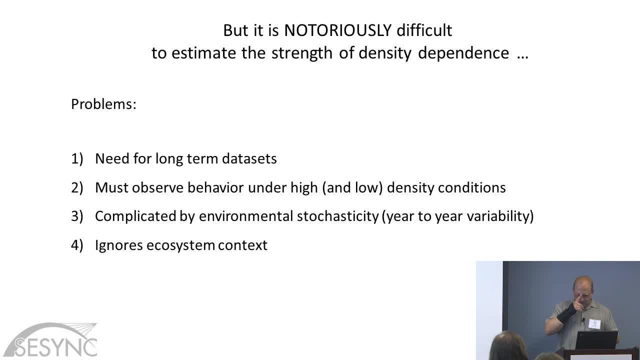 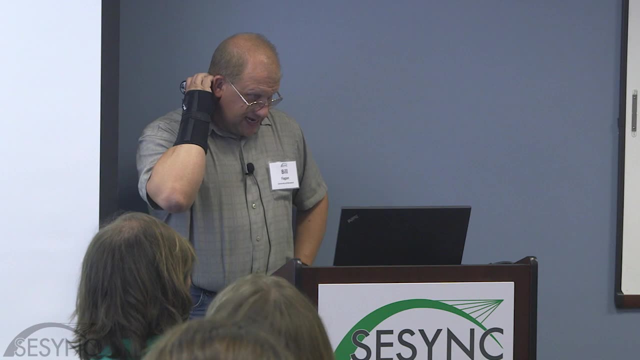 might bear on it. We don't have that kind of information, And so we have all kinds of problems that lead collectively to this problem of estimating density dependence. So one partial solution- this gets to the work that Olaf and I are doing together- is the idea of what are 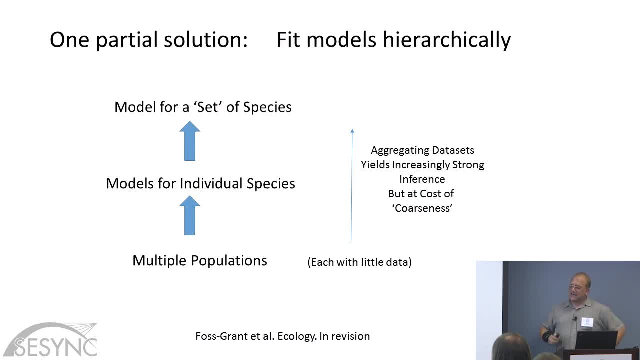 called hierarchical models, And the idea is that if you're struggling with data, sometimes by aggregating the data together you can get really good information about a question that's related to the one that you're most interested in, but not exactly because you have to ask the question. 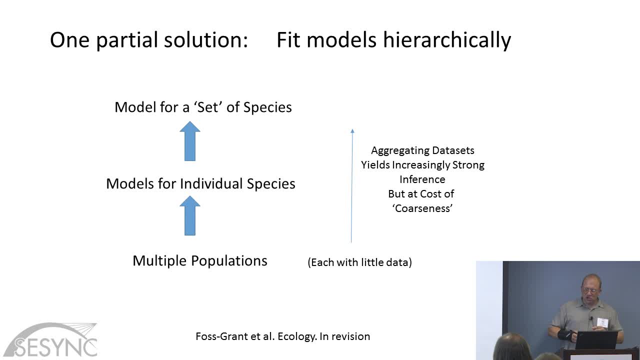 at a different scale, And so, in the case of fisheries assessments, you can think of a hierarchical model that's related to the one that you're most interested in, but not exactly of organization being out there, And in this case you have multiple populations of the same. 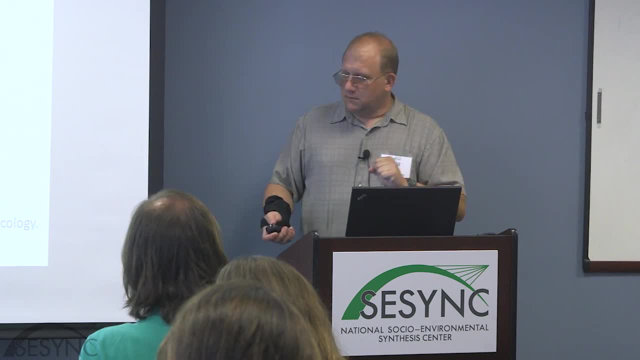 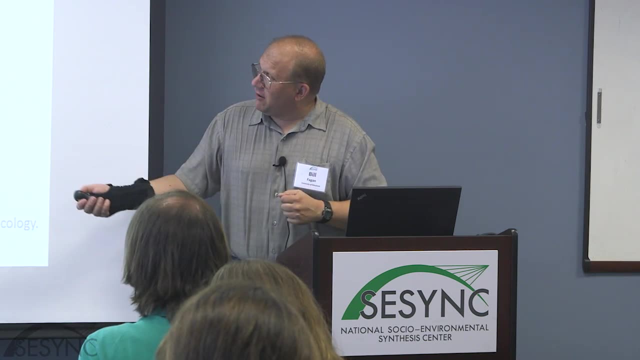 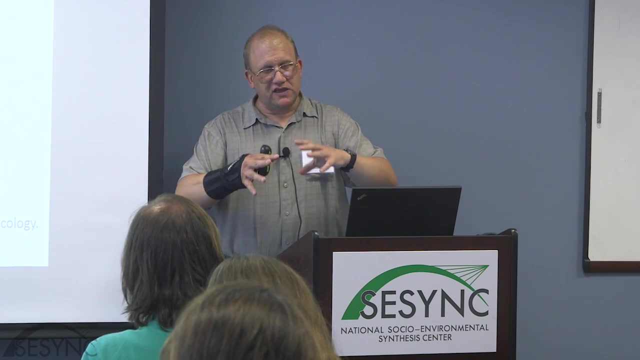 species of fish. The same fish might live in different water basins, for example, but in each case you only have relatively little data. But we can aggregate those data together into a model for the individual species that brings together the information from the different water basins. 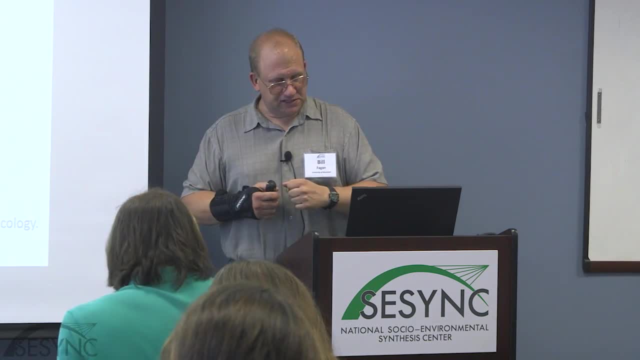 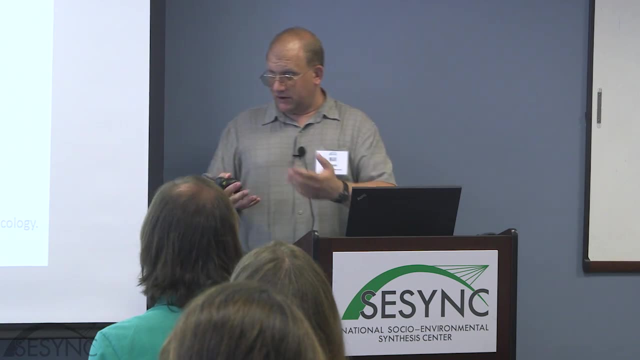 to say something about the level of the individual species, And we can go further than that to say that we've got a bunch of related species that are similar to one another, that, by virtue of their evolutionary history, might be able to respond in a similar way, And so we can add something. 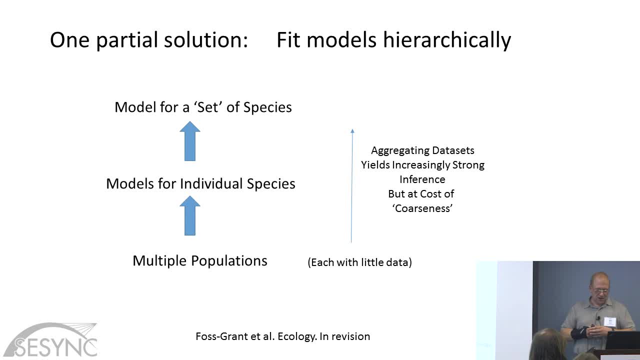 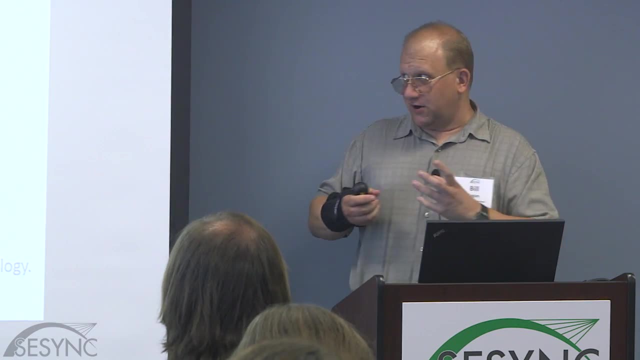 at another level up here to have a set of species, And as we aggregate data we become more and more confident. The data set becomes more and more robust in our ability to say things. but it comes at a cost, because the cost here is the coarseness of the question that we 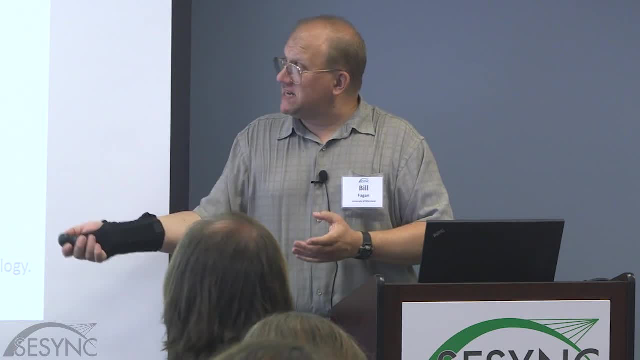 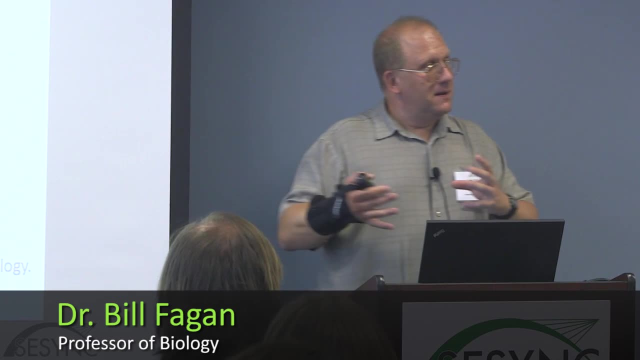 can answer with that aggregated data. We might have relatively little data to ask a particular population-level question, but as we go up and up we're adding data but we're no longer in a position to answer questions at the level of the population. We can only work at this more. 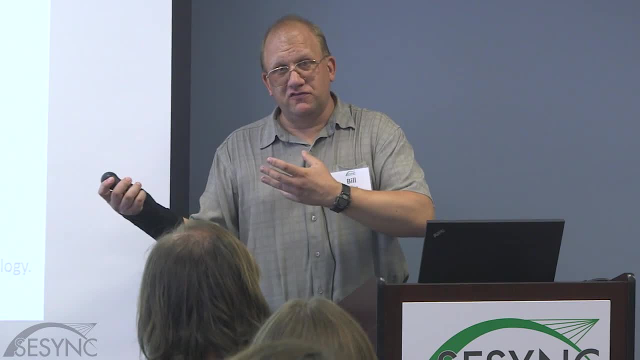 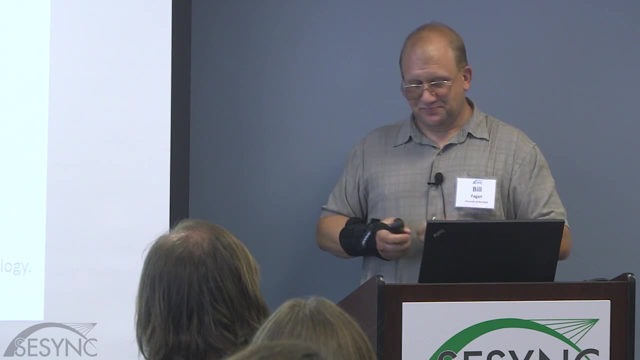 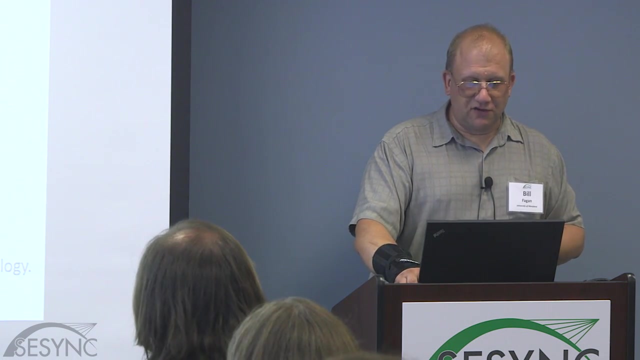 coarse scale, And so this is a transition, It's a trade-off, but this idea of aggregating information in a hierarchical way has virtue, And so, for example, if we build models- statistical models in this case- that are fit hierarchically, we can, for example, 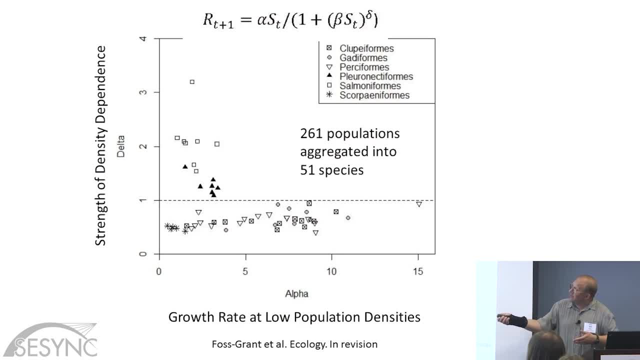 take 261 fish populations, aggregate them into 51 species and then say something about the population dynamics of those 51 species. And you can see, here there's the 51 species. And you can see, here there's the population dynamics of those 51 species. And you can see, here there's the 51 species. And you can see, here there's the 51 species And there's the 51 species And there's the 51 species. There's the 51 species that are coded. 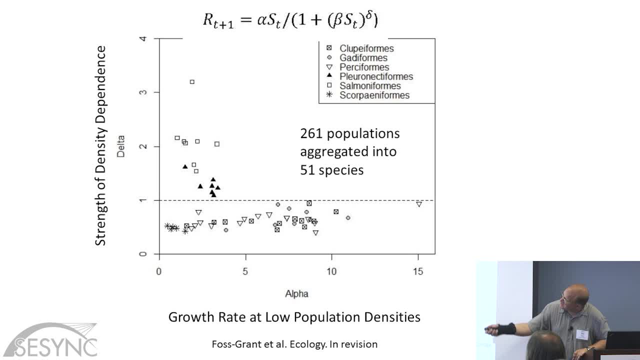 by these symbols here and this axis here is the strength-of-density-dependence, that's that delta parameter, And on this axis is another parameter, alpha, which governs how quickly the population can grow from low densities. And you can see that there's kind of a clustering. 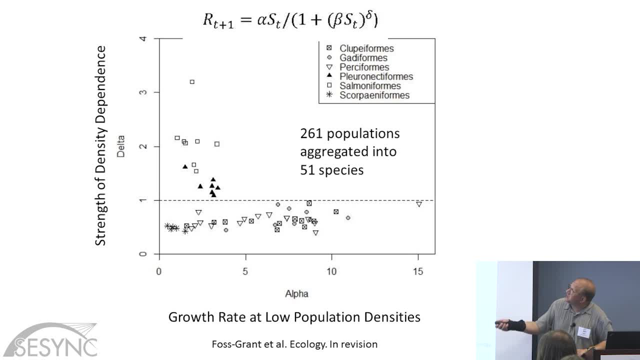 in some places where, for example, these six species are all members of the pleuronecteiformes, They all have the same kind of response, same kind of underlying parametric structure to their population dynamics. The same is true for the salmon that are up here. They all 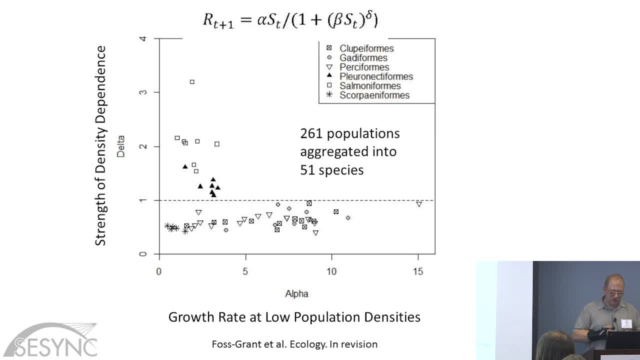 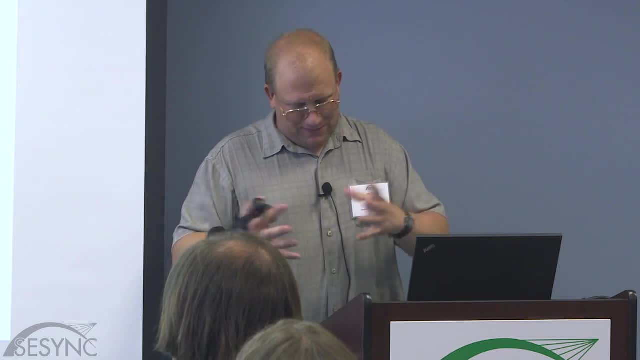 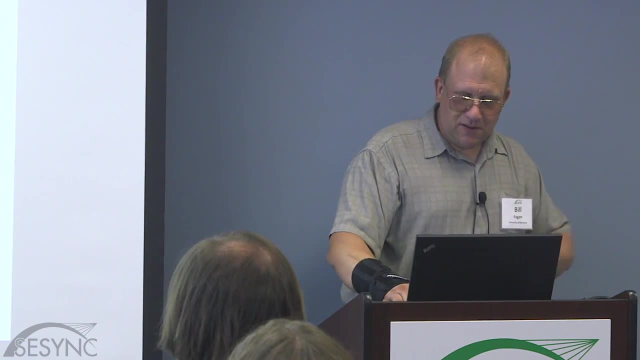 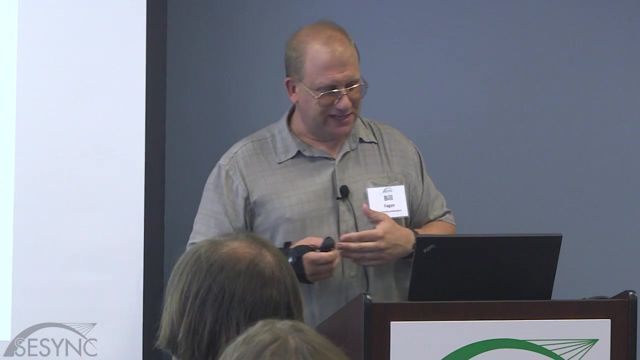 have these very strongly density dependent behaviors. And so we're able to say things about populations by virtue of aggregating, we're able to say things about species by virtue of aggregating data across many different populations of that species, And then, at the next level, we can say: how do the different orders of species behave with respect to density? 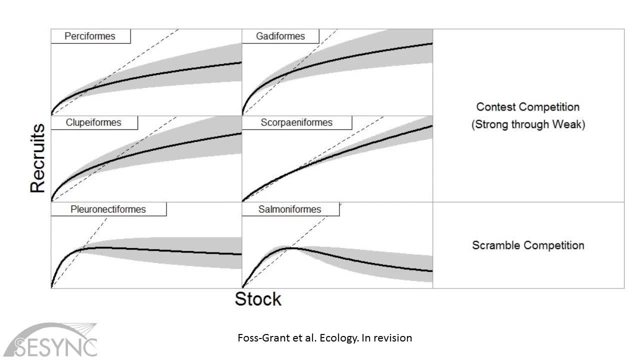 dependence And we can see that there's very different response curves here for the stock recruitment dynamics of these six different orders. These here have contest competition, whether in some cases it's very strong contest competition or weak. But in these two groups you have strong evidence for scramble competition. We think in this case, in these two cases, 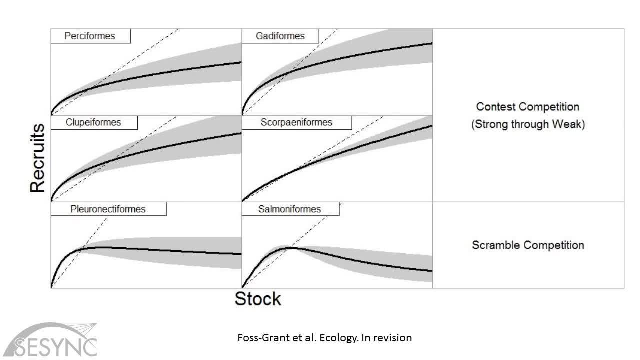 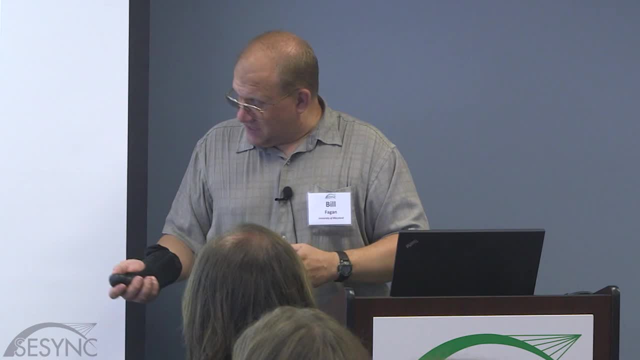 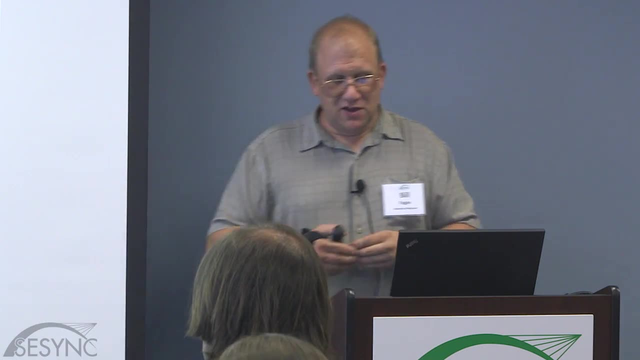 it's mediated through their competition for spatial resources, like the reds, the stream bed egg masses that salmon have. But the idea is that we're aggregating information and being able to say things at these higher levels that might be useful from a management. 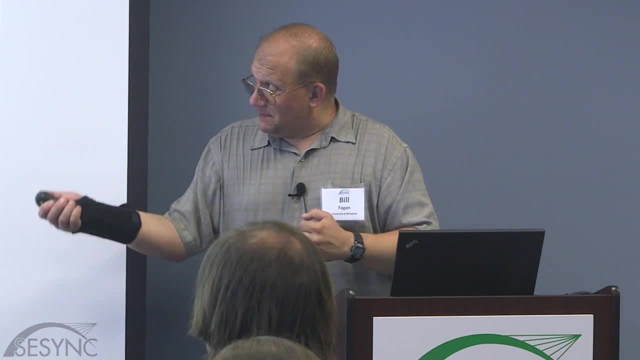 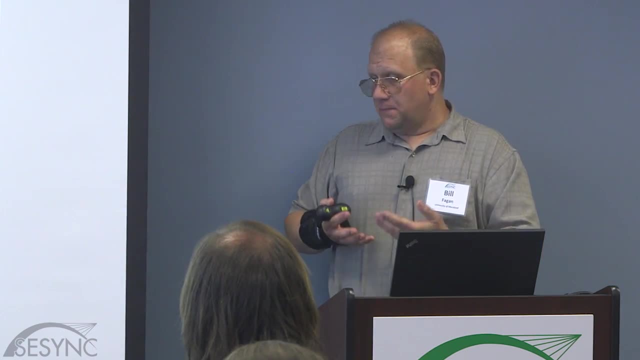 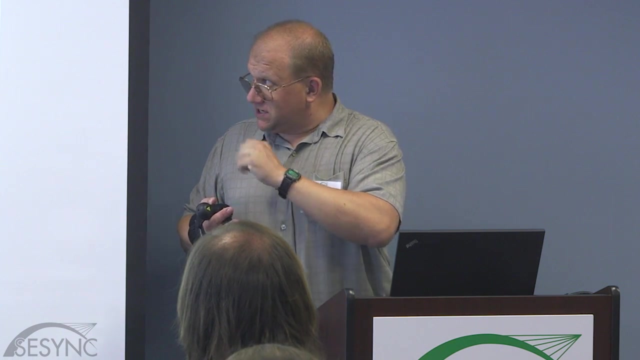 perspective, For example. in this kind of a setup we have an empirical starting point then for choosing one kind of model as opposed to another, because we know that you know that evidence for density dependence is going to differ across the different groups. We 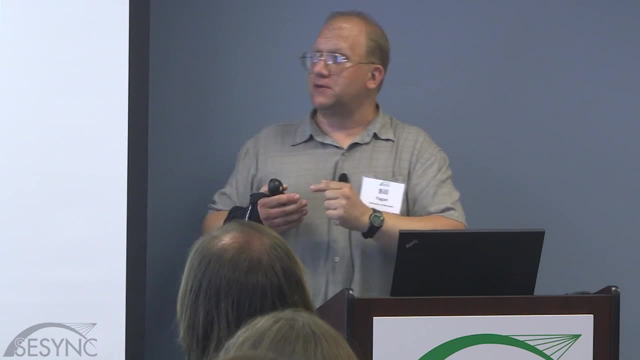 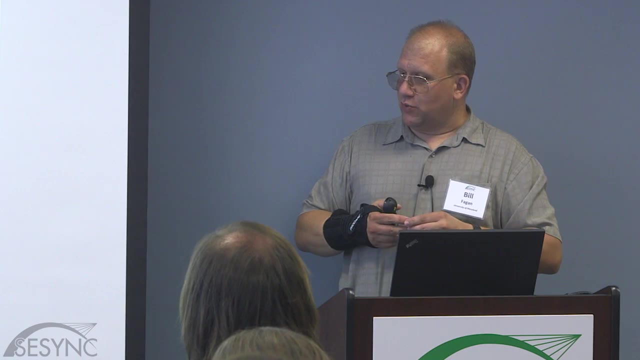 wouldn't have known that if we had only looked at each population individually. Aggregating the information and then working upwards in a hierarchical way allows us to answer different questions at these different levels of organization, And we can think about that as a resource. 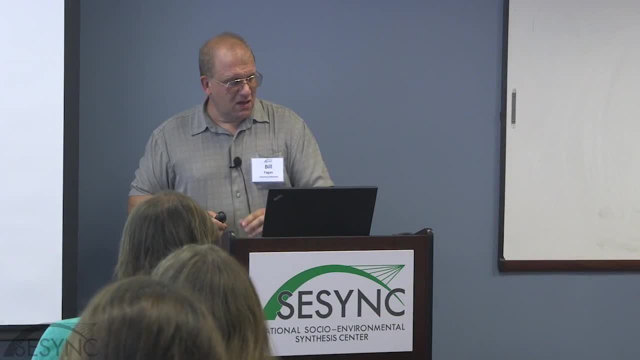 an approach that might be useful in other contexts. Okay, And then the last way we can reach this sort of answers is through different ways. One way we can get this answers sort of from the network of action maps. So at the very beginning I had the right idea to come. and the result is is that we can look at a very narrow bottom In the search capsule. we'll get an idea if we, if you look at the data you get from the disk and you have a view of the data. 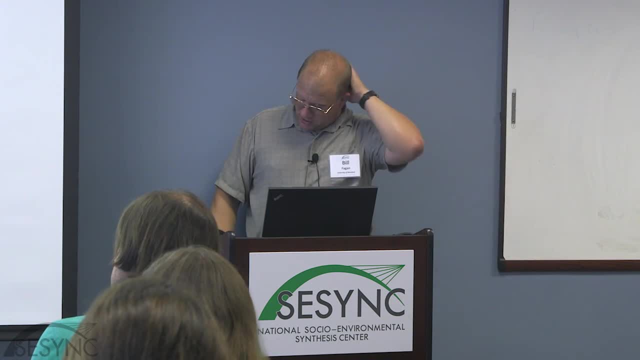 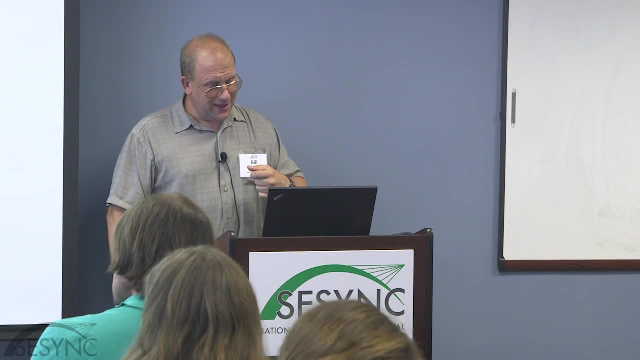 Next two basic principles that Berryman talks about are interactions with other species, which take us to community ecology, so I'm not going to belabor that today. And then the last one I really like, especially in the context of general laws of ecology: 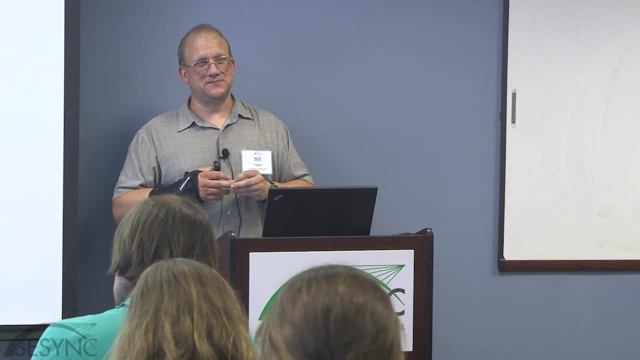 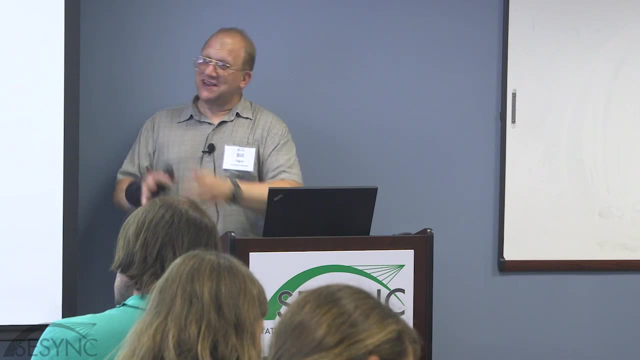 the idea is that limiting factors change in time and space, And what this means is that all of the preceding four principles that we've been focusing on are really context-dependent. So I mean, it's kind of a non-sequitur, but I find it interesting that we can talk about